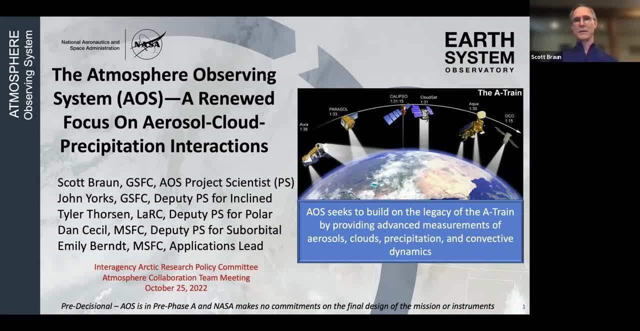 convection and precipitation, And so this mission is the means by which we are trying to implement those designated observables, And the people shown here are the project science team, including Emily, who will talk about applications right after me, And I only plan for about 10, you know, maybe around. 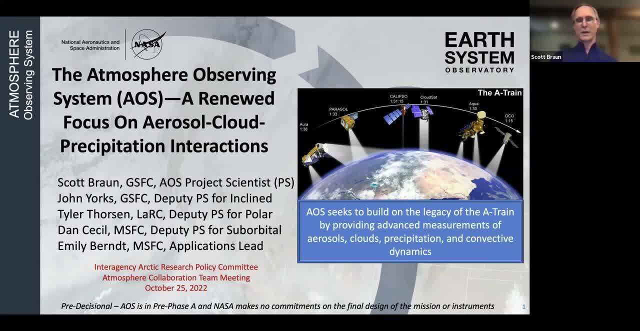 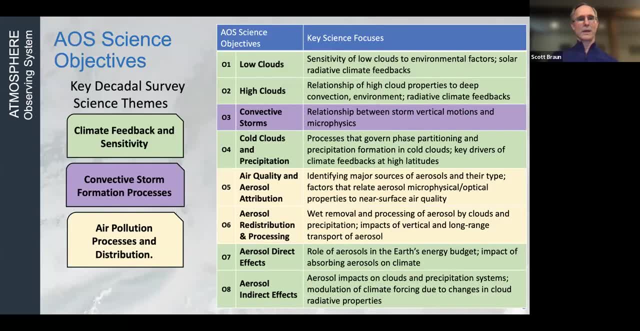 12 minutes of presentation. I wanted to build in enough time for questions and discussion, particularly at the end. So if you have a question, you can go ahead and interrupt me. I just want to give you a high-level overview of the science of AOS. The Takedo survey had identified a number of science objectives related to 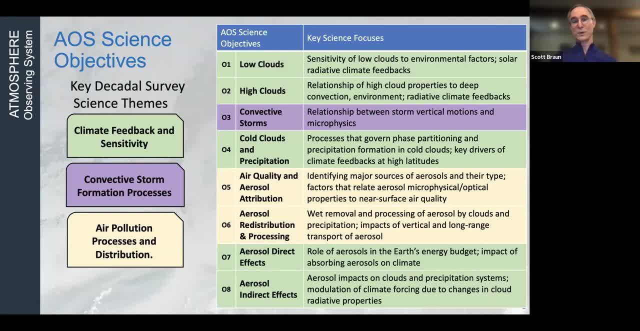 aerosols and clouds, convection and precipitation, or CCP, And many of these fit within three main themes, which are climate feedback and sensitivity, convective storm formation processes and air pollution processes and distributions. And our team, in a study that we did from late 2018 to early 21, looking at 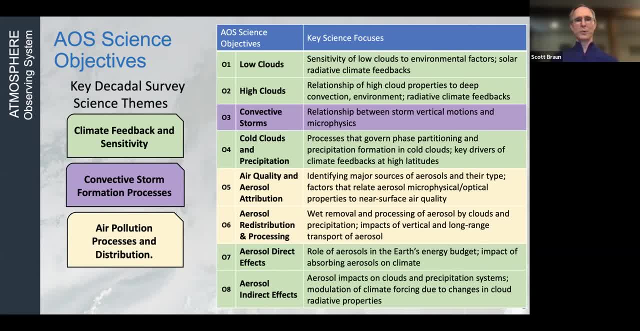 architectures. we sort of pulled those objectives together and tried to find ones that we thought we could implement, And we found that there were a number of themes that we could implement, a specific set of objectives that follow those themes. And so in the green, which is the climate feedback and sensitivity, we have cloud feedbacks. 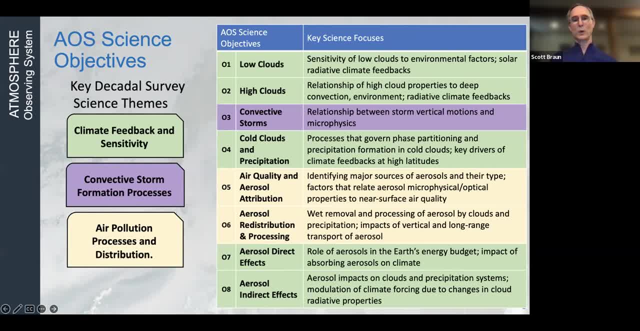 as identified in terms of high and low clouds and cold clouds, So more or less polar clouds where you have mixed phase or frozen clouds near the surface, And then aerosol direct and indirect effects. Convective storms is kind of on its own side. It's focused on relating convective storm microphysical properties to the dynamics. 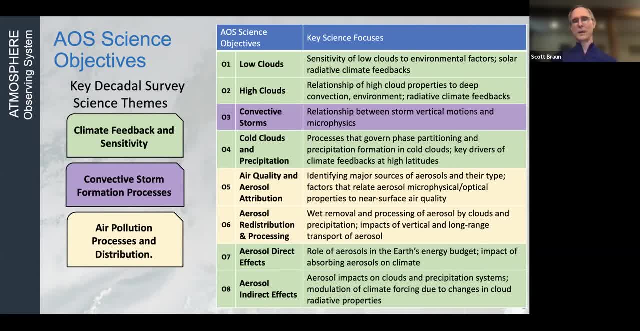 of those storms, with the dynamics coming from Doppler radars, And then the aerosol objectives, which are focused on aerosol properties and profiles as well as aerosol movement through the atmosphere, So from emission to short and long-range transport and eventual removal. 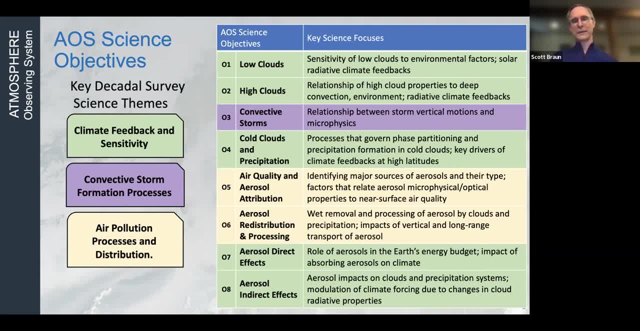 Okay, And we used those objectives as the basis for identifying what geophysical variables are needed to answer those objectives or address those objectives. That formed the basis of a science traceability matrix And ultimately, we flowed the need for those geophysical variables to a set of measurements and built the architecture by looking at a range of instrument capabilities. 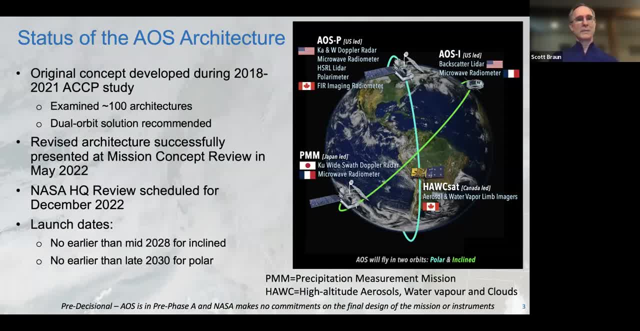 that could address those measurement needs And, as I mentioned, so from late 2018 to early 2021, we did this architecture study using – we had put out an RFI to collect information about a variety of technologies that were available in the – that were expected to be relatively mature by the early to mid part. 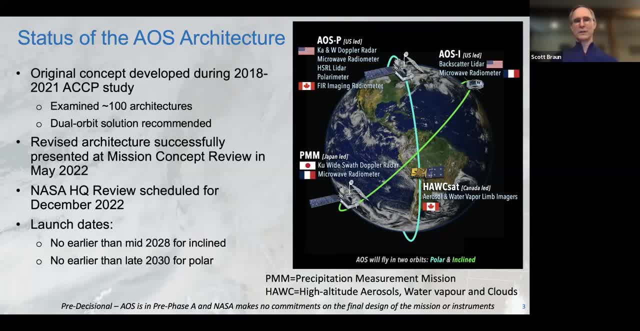 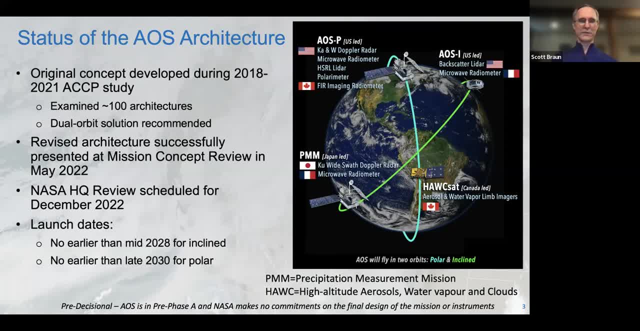 assessments of the quality of the observations that would come from the different instruments, And we eventually whittled that down to an architecture that headquarters accepted. It was a dual orbit architecture similar to what's shown here, So an inclined orbit to go after dynamically varying processes, particularly if you're focused on convection and high 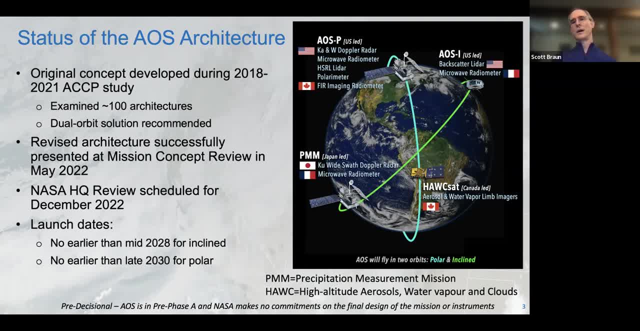 clouds. you know that has a very strong dynamo component And that's what this mission – that project is targeted for. And then a polar observatory, which is really geared toward globally distributed observations and geared toward the highest quality measurements that we could provide and noting that we really wanted synergy of those measurements to get. 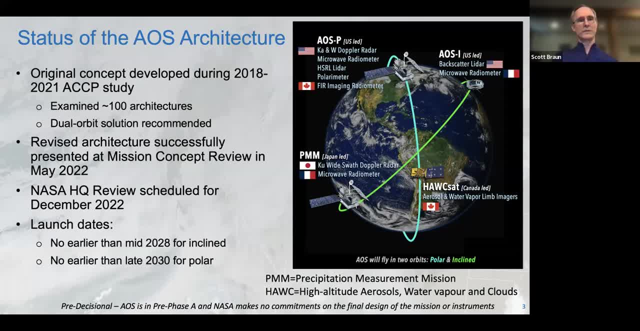 the best possible estimates of these geophysical variables. We took that architecture through pre-formulation over the last year or so. We had to make some descopes as costs increased. And then we took that architecture through pre-formulation over the last year or so. We had to make some descopes as costs increased And then we had 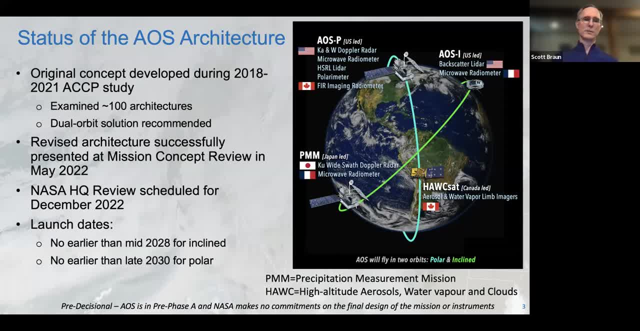 to make some descopes as costs increased. And then we had to make some descopes as costs grew and tallying that cost as we refined the cost and the overall costs went higher. most of the descopes went to the inclined project, not the polar, And then the concept. 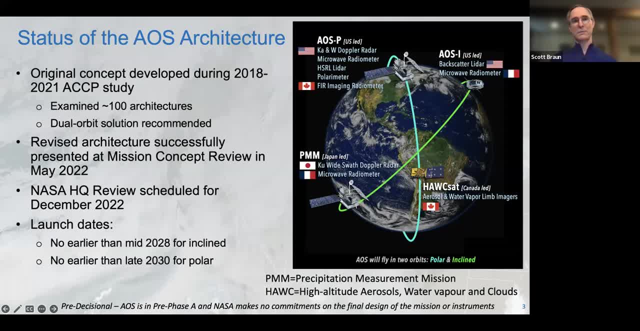 that's shown here is what we took to our mission concept – our concept review in May, which we readily passed. So this is the architecture we're moving forward with. now We're getting ready to move toward our key decision point: A review in December. 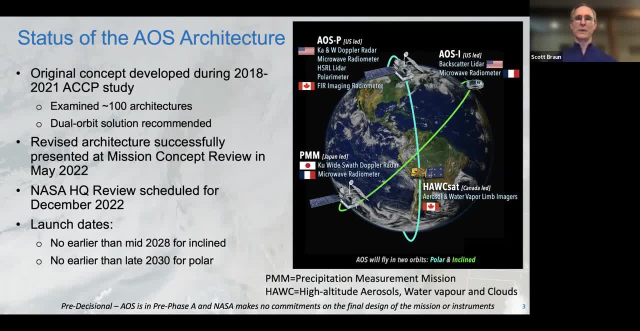 Are we all ready? headquarters had started up an independent review board to assess all the designated observable missions. They've received the recommendations from that IRB and they're still evaluating those. So we haven't heard whether there are going to be recommended changes to the architecture. 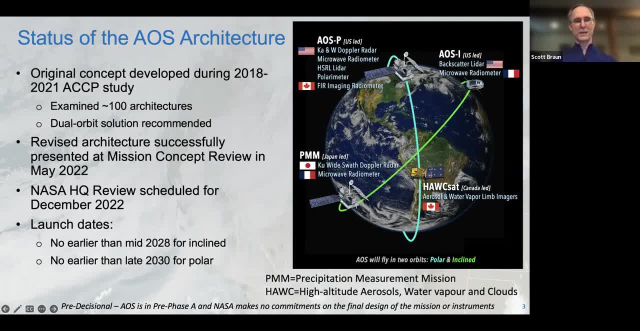 It's certainly possible and that's why you'll see down at the bottom here where we say it's pre-decisional, There are. it's possible that some aspects of this architecture could change. I'm not going to talk about the inclined orbit later. 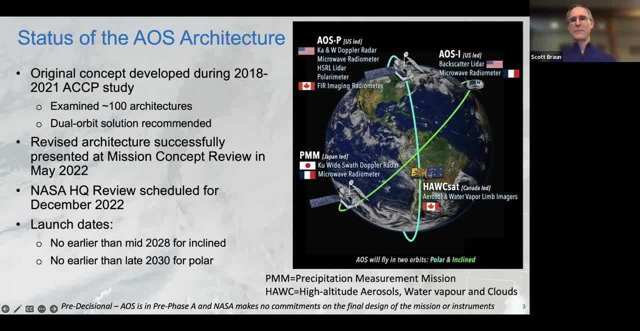 in this talk, so I'll just briefly summarize it here. It includes a JAXA KU band wide swath precipitation radar with nadir Doppler capability. That's on one spacecraft. a Japanese observatory- The NASA observatory- will have a backscatter lidar. 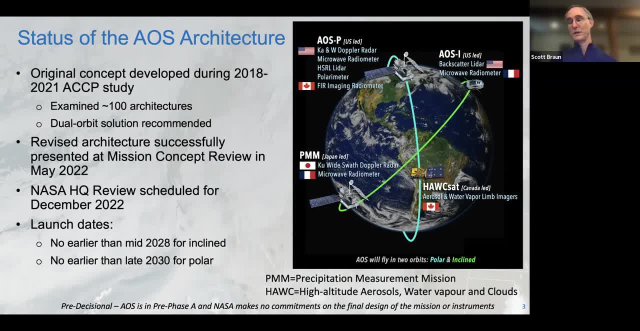 that's comparable in capability to Calypso, but in a smaller, more affordable package. And then on both- both of the satellites- we will have microwave radiometers with frequencies ranging from 89 to 325 gigahertz, And those will be separated by about two minutes. 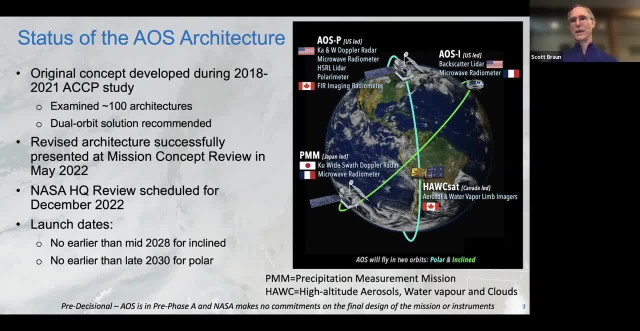 And the goal there is not only to characterize high clouds and, to some extent, precipitation processes, but using the time rate of change of the brightness temperatures to infer something about the dynamics of the storms, given that the change in brightness temperature changed, you know. 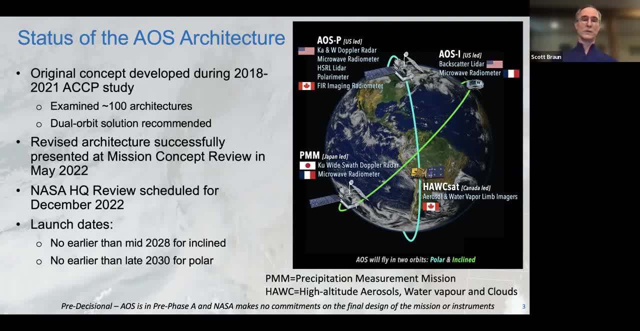 temperature reflects a change in the microphysics over that short time period. that tells you something about the vertical ice mass flux within the storms. The polar capabilities I'll describe in the slides that are coming up and I'll just note that the inclined orbit is going to launch. 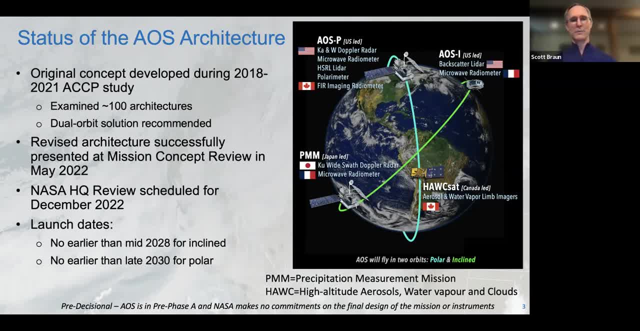 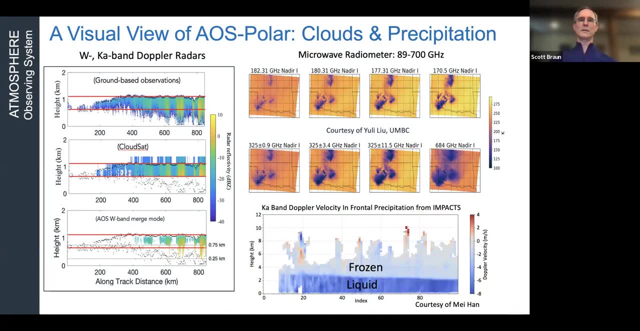 no earlier than mid-2028 and the polar component would be no earlier than late 2030.. So let's talk a bit about some of the capabilities in polar, and we'll start with clouds and precipitation. We have a couple instruments here to highlight. One is a Doppler radar that is expected. 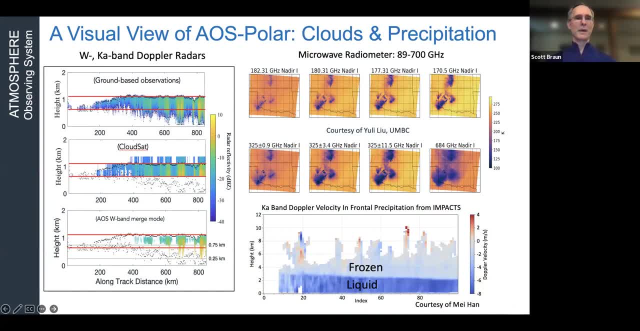 to be built by JPL. It's W band and Ka band. The W band is sort of similar to CloudSat in being able to profile clouds, but it doesn't have the exact same capabilities. We made some trades, due to a number of reasons, in trying to advance the science in some ways and then being 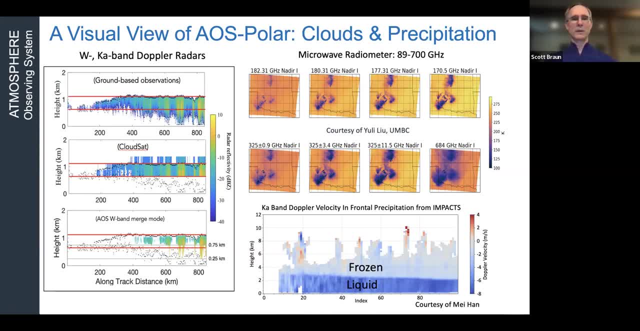 cost constrained in others, but one of the things that we really wanted to do was to be able to sample closer to the surface and just to give an example here on the left, this: these are low clouds as observed by a ground-based radar, and you can see the cloud tops are just above one kilometer. 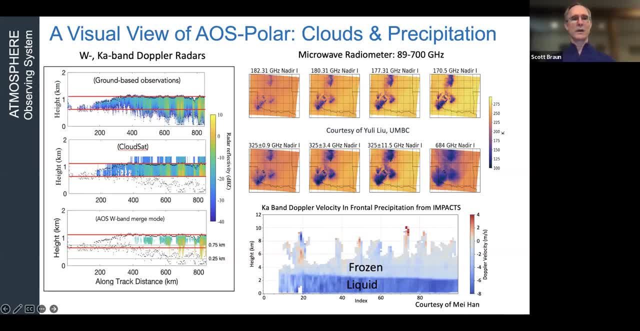 Cloud base varies from about 700 meters and then lower, and you have some areas of precipitation within the cloud. This is a simulation of what CloudSat would see, So because of its coarse vertical resolution, you get some pixels extending the cloud vertically when it's actually above cloud top The cloud. the cloud boundaries are indicated by these dots. 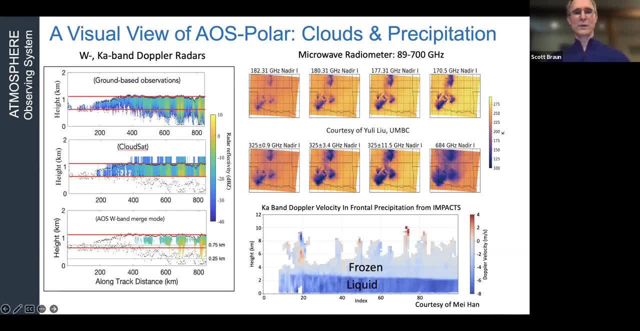 There are about two range gates within the cloud and then, due to surface clutter effects, you end up with this blind zone down low where you can't see what happens in the lower layers, Whereas with the mass radar we sacrifice a bit of sensitivity, at least down low, to be able to profile closer to. 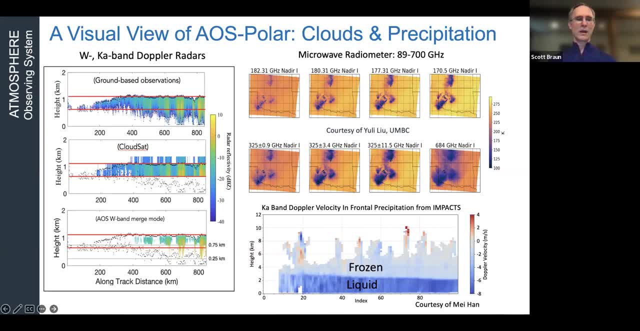 the surface. So we're primarily seeing areas of very light precipitation, very fine vertical resolution of a few hundred meters and in, and then you can also see down to about 300 meters or so, these precipitation shafts, Once we get above the boundary layer, the sensitivity 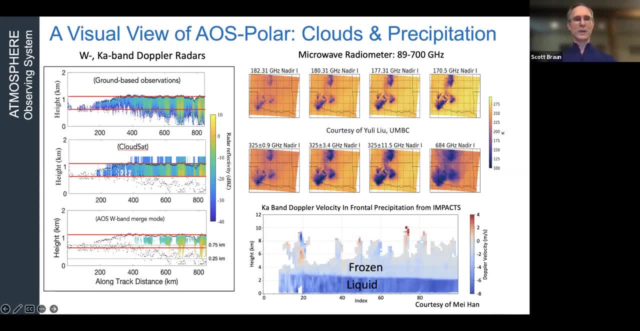 improves quite a bit- Still less than CloudSat, but not nearly as bad as what you see in the lowest one kilometer. And again, this is just due to surface clutter effects that make profiling in the boundary layer quite difficult. Now, from a precipitation standpoint, 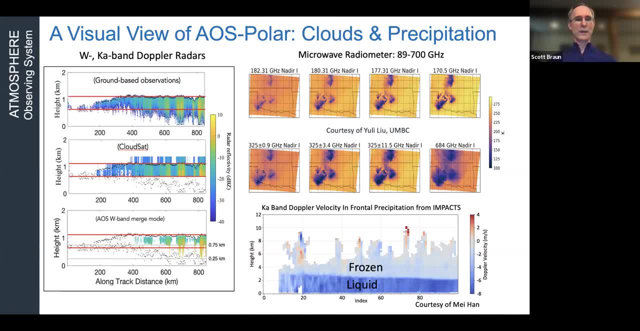 in particular, snowfall. this W-band radar is going to be great because you're generally going to have higher reflectivities and we will get profiles down to a few hundred meters, So your radar will be much shallower than it would be with CloudSat and other typical radars. It'll be 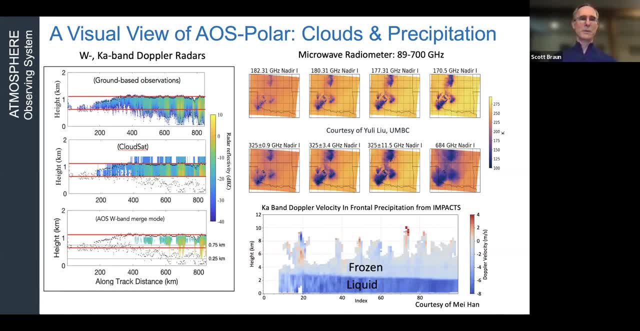 good vertical resolution and by having W-band combined with Ka band, we will be able to get some estimates of the particle sizes using dual frequency approaches. Now, both of these radars will be will have doppler capability, using what's called the display space center antenna approach. 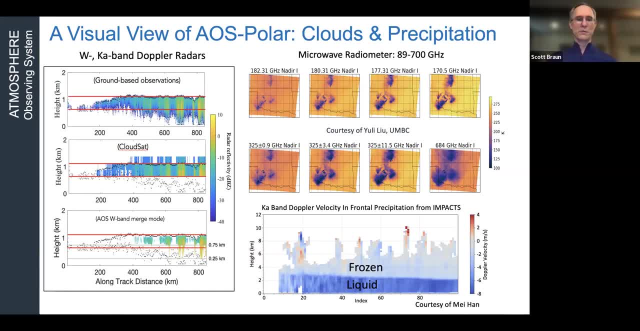 It's basically, instead of one antenna it's two and that helps to remove errors associated with the spacecraft motion and non-uniform beam filling. And I'm just using an example here. it's actually radar data from the impacts airborne campaign for the Ka band frequency and it's been degraded in resolution to be kind of comparable to the AOS. 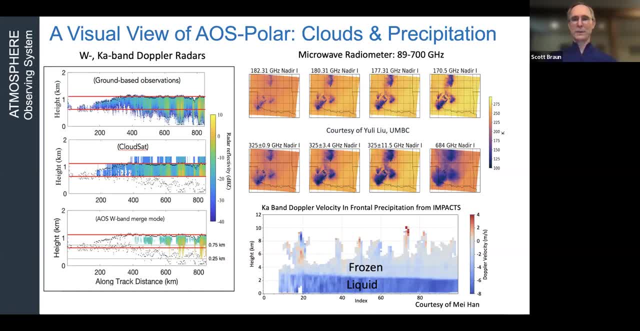 resolution, But you'll be able to see, through the doppler data phase, changes from frozen precip to liquid And with the improved doppler accuracy we'll be able to see some of the vertical motions, for example when there's embedded convection. In this case, there was this elevated convection above the, the frontal zone in this snow event or well. 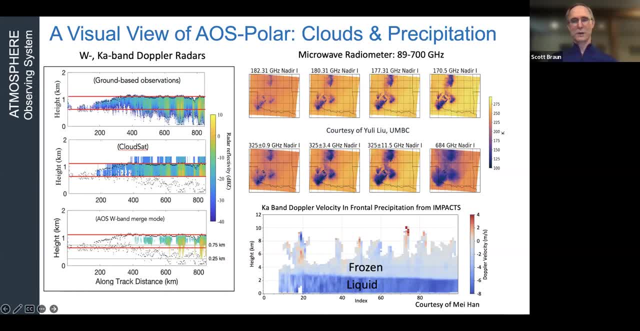 rain event. It was snow elsewhere in the storm, But that kind of gives you a sense of the capabilities we'll have from a doppler perspective. And then up in the upper right is an example of the passive microwave data. We'll have frequencies in the polar orbit from 89 to 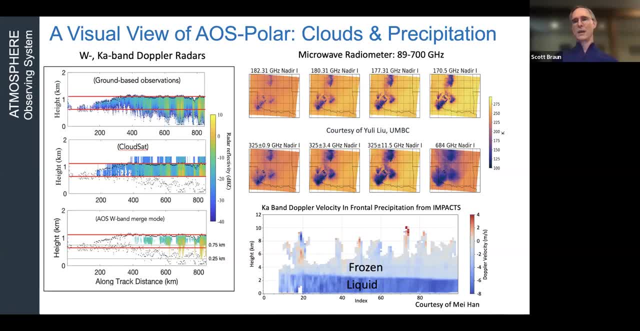 2.5.. to 700 gigahertz, primarily 89 or 113, 183, 325 and then 640 to 700. we're hoping also to get channels near like about 160 to 240 for better measurement of snowfall at the surface, at least at mid. 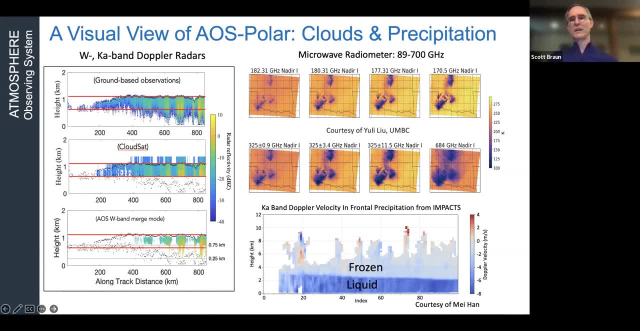 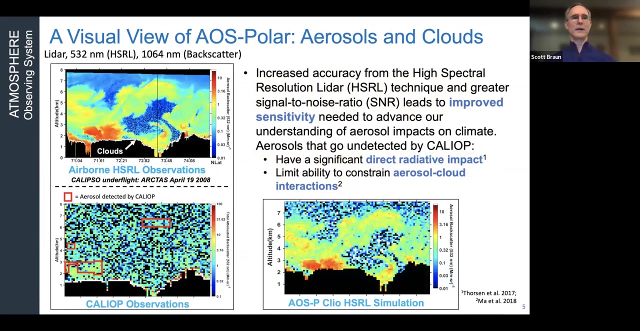 latitudes and this is a sim. it's a simulation of a convective system, but you can see how the scattering by the ice particles varies by frequency, where typically you can distinguish the more intense ice amounts at these lower frequencies. but you need these higher frequencies to see the full extent of the cloud shield. this is an example from the lidar, so the lidar will. 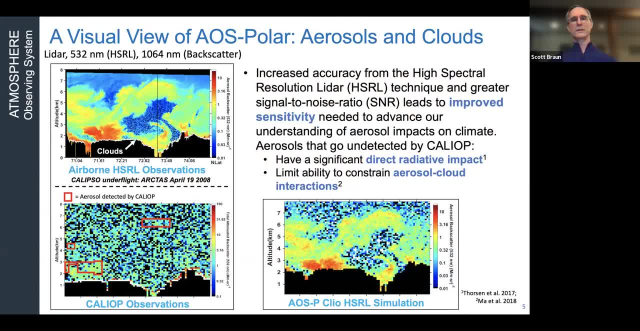 have two wavelengths at 532 nanometers. we're expecting it to be a high spectral resolution lidar um, which means it has an hsrl filter that helps you to separate the particulate backscatter from the molecular backscatter, and then we'll have a backscatter channel at 1064.. there are many. 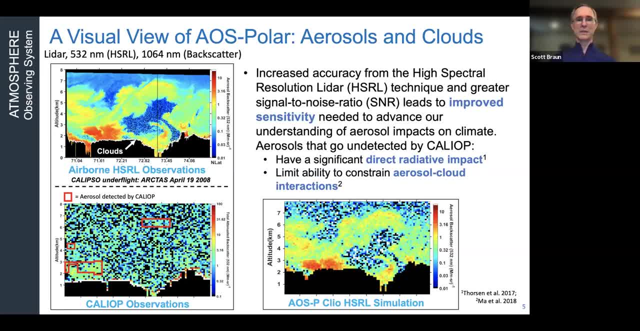 advantages to having that hsrl. we expect to have much better signal to noise than calypso. but with the, with the backscatter lidar, you're basically solving for two unknowns with one equation. so it's an under constrained problem and you have to make some. 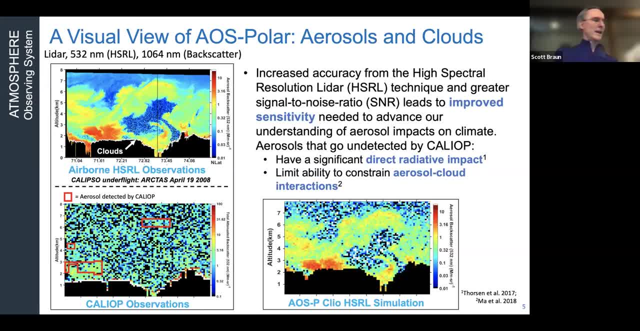 assumptions, uh about the, the ratio of the backscatter to extinction with the hsrl. you're basically getting two pieces of information, two equations for two unknowns, so you can get a much more accurate uh: retrieval of the aerosol, total particulate backscatter and extinction: uh, including in situations where there's at least then. 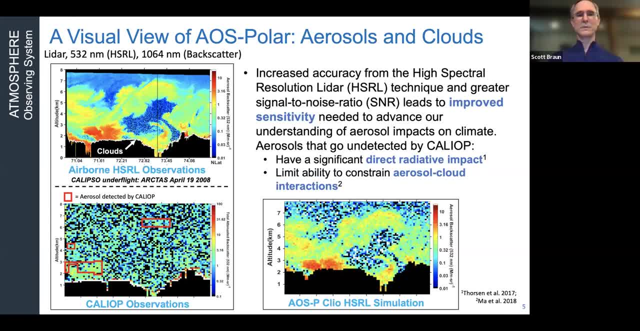 overlying clouds, which is a problematic area for calypso. we also expect to have to do uh, tenuous or faint aerosol much better, and the example that's shown here is airborne data in the upper left from an experiment that was in the arctic region. you. 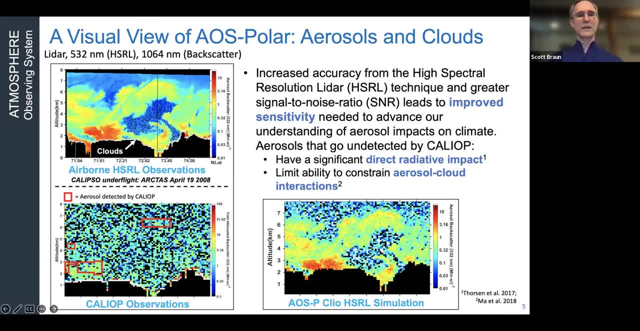 can see the the latitudes here, ranging from about 71 to 74 or 5 degrees and showing aerosol over a cloud layer, and you can see some more intense aerosol and then these very faint aerosol layers. this is what calypso saw. in this event, you can sort of make out. 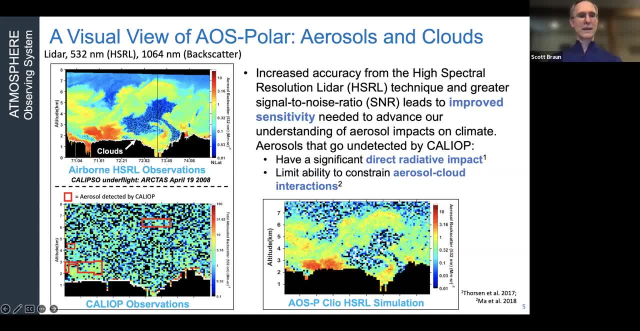 this aerosol layer here, but, and the boxes indicate uh areas that were identified by the calypso algorithm. but there's a lot of noise and pretty weak signal and this is a simulation that langley did of the hsrl instrument from space and you can see it does a much better job. 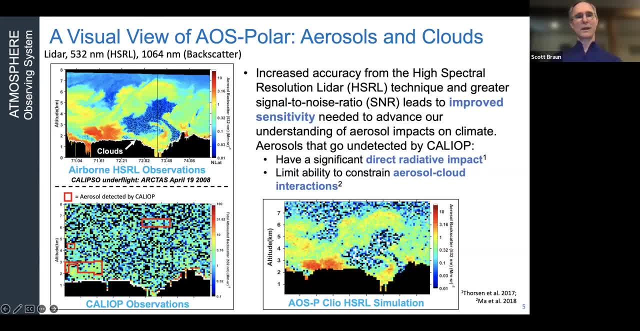 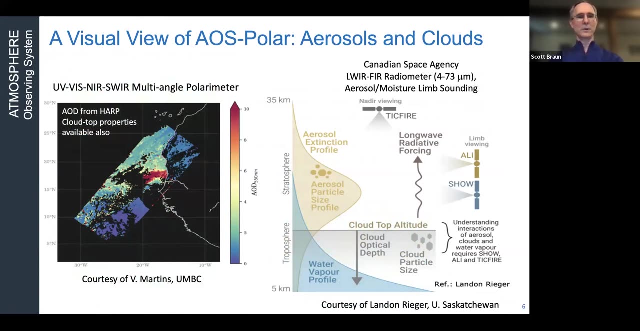 of detecting and quantifying the aerosols in this region and this will be very useful for looking at the direct radiative impacts of these faint aerosol layers and can also be important if you're looking at cloud aerosol interactions. a few other instruments in this polar orbit. one is a multi-wavelength, multi-angle. 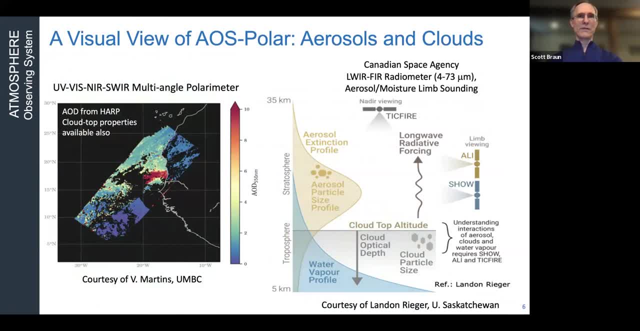 polarimeter. this will allow for fairly accurate retrievals of aerosol optical depth absorption and particle size, and also at one of the wavelengths. with the multi-angles you get cloud bow measurements, which gives you information on cloud particle phase and particle size and variance. the swath is expected to be at least. 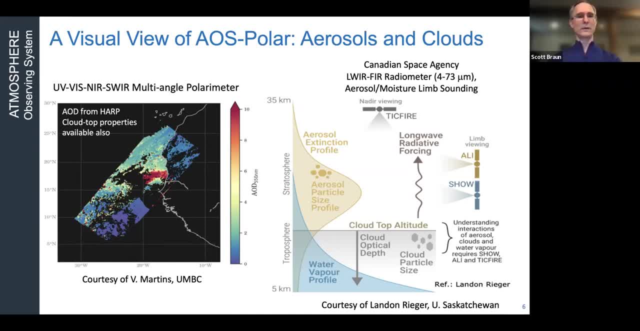 300 kilometers. we're certainly hoping to get it a bit wider, and this is just an example of aod from the harp instrument, but it's at least conceptually similar to what we would expect to get from aos. and not only will the the polarimeter observations by themselves. 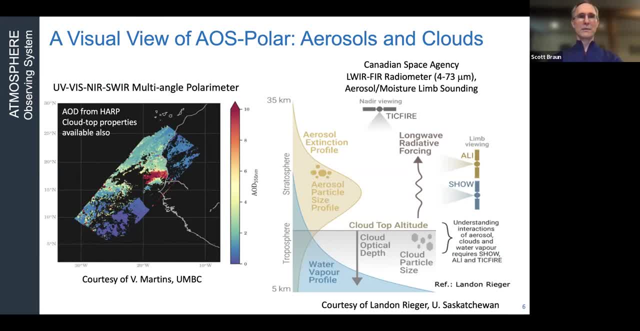 have a lot of value, but we are anticipating having combined polarimeter lidar retrievals that use the best information from both sensors to get the best retrievals. and then from the canadian space agency we have a long wave and far infrared imaging radiometer that will be on the same spacecraft as the instruments i was just talking about. they'll 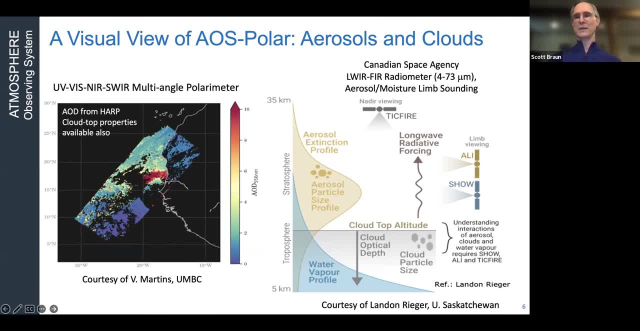 all be looking down and then on a csa provided spacecraft, they'll have two limb imaging uh sensors, one for aerosols and one for moisture, that will help to characterize the upper tropospheric lower stratospheric water vapor and aerosol properties that spacecraft will. 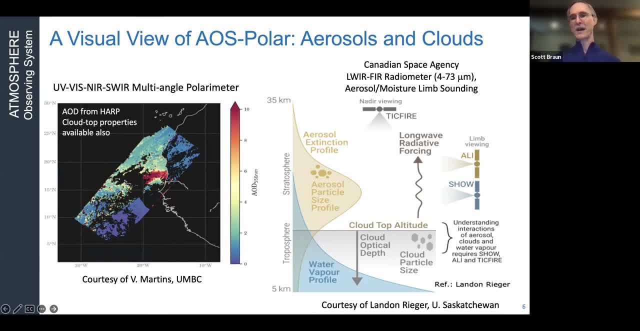 be following the, the larger spacecraft by about five minutes due to the geometry of the viewing, and, and so from tick fire we'll get uh, cloud optical depth and cloud particle size information, as well as some information on uh long wave radiative forcing, uh, and again with the ali, you get the aerosol extinction profile and information on particle size and so on. 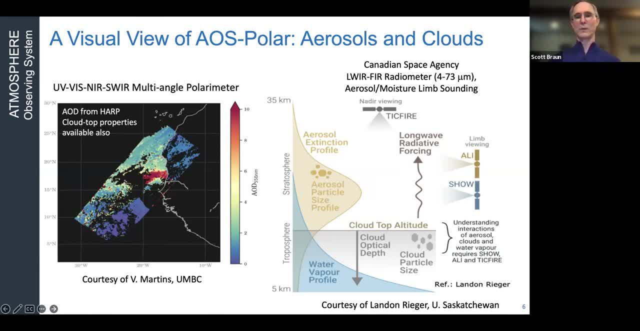 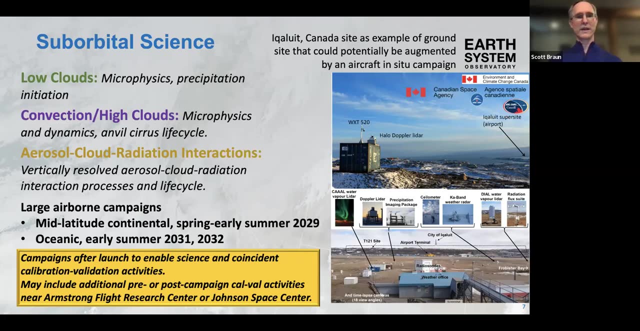 and this information will be great to have in combination with the lidar and the radar in terms of connecting the cloud processes with these aerosol and moisture processes. we're also going to have a suborbital campaign that will focus on low clouds, convection, high clouds and aerosol cloud interactions. these campaigns are sort of 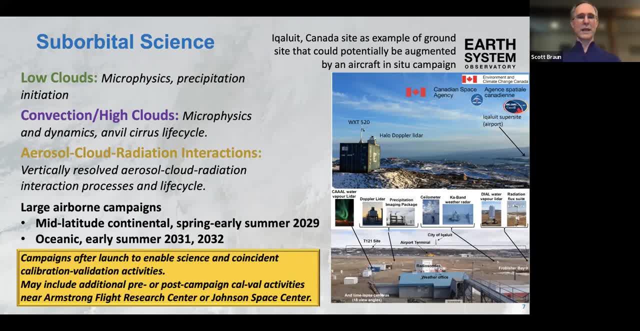 earth venture suborbital type. if you're familiar with those, you know really large campaigns, probably three of them spanning the years after the launch of the two projects in the mission. most of these will probably not be in the arctic region, but we have been looking at using data from a ground site at qualiwag, canada, and we're considering the possibility. 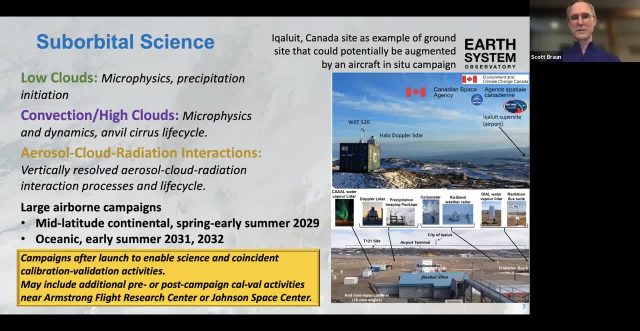 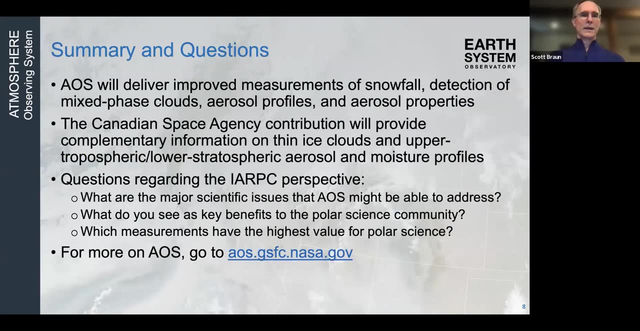 of at least maybe a limited airborne campaign, maybe just a single aircraft with a limited set of instruments, where we could have combined there the airborne and ground-based data. but that's still to be defined in the years ahead. so in summary here, uh, yeah, i think aos will deliver improved measurements for 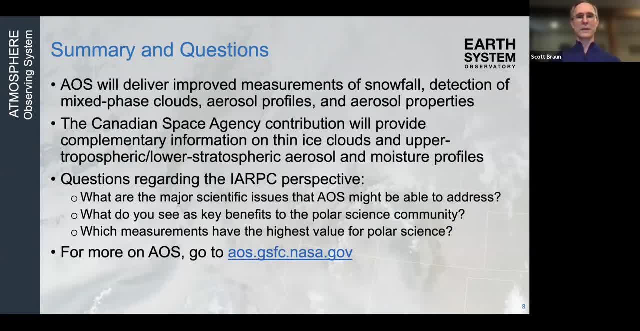 snowfall with the dual frequency radar, detection of mixed phase clouds from the polarimeter and the lidar, and then the aerosol profiles and properties from the polarimeter and lidar, as well as with some of the csa instruments- and i'm really excited about the csa uh contribution. 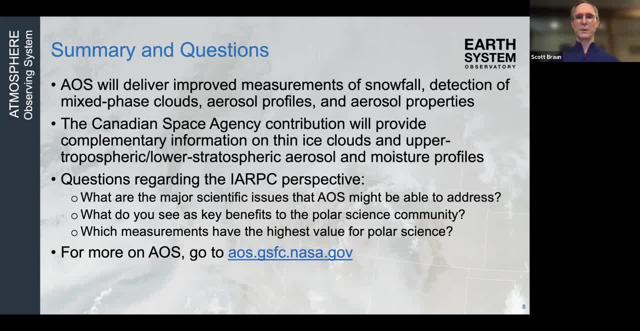 to this uh mission. i think it really helps to fill in some gaps, particularly related to the upper troposphere, lower stratosphere. that'll be a high interest, certainly to the convection community, but i'm sure to many other communities as well. uh and i. i would imagine you have questions for me. 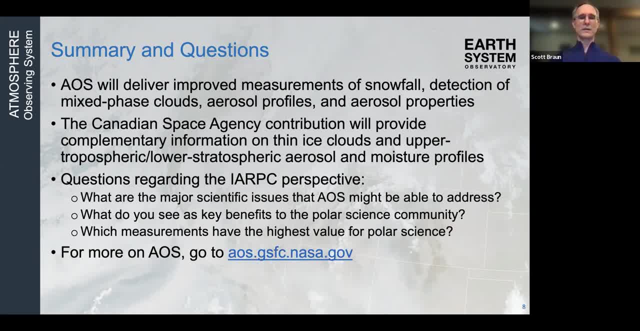 but i have some questions for you as well in terms of what some of the major scientific issues are that aos might be able to help address, what you see as some of the key benefits and maybe what measurements uh are viewed as having the highest value uh to arctic science. so with that i'll stop. 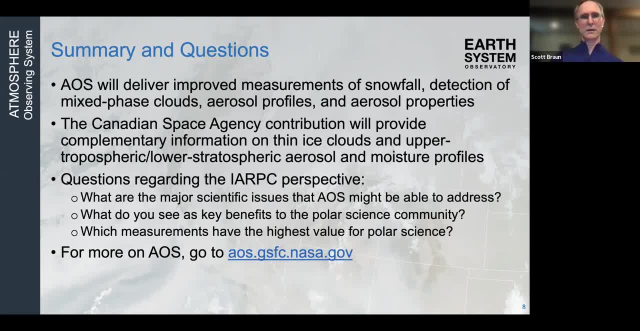 there and, and maybe before we go to emily, we can see if there's, if there are, any questions that you might want to ask before we move on to the presentation. um scott, this is david romwich. um, one question that i have is the repeat time of the measurements. 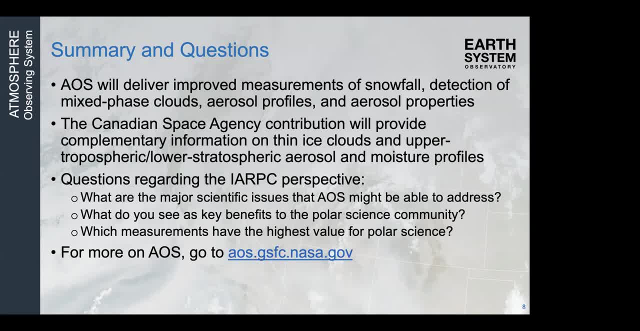 these seem to be relatively narrow swath instruments. see, can you talk about that please? yeah, we haven't settled on the exact repeat time it'll. it might end up being comparable to cloud set and clip. so so a lot of these measurements are um nadir or near nadir. uh, at least the active. 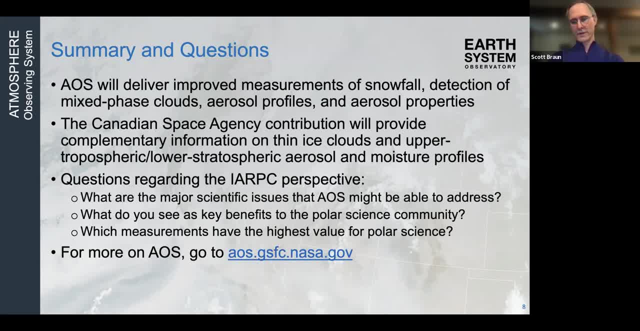 like you're trying to get broad coverage of the observations. over time, you, you want to sample more of the globe, and so the trade-off is, uh, getting broader coverage and making sure you don't have holes. if you're trying to aggregate data, uh like on a monthly time scale, you don't. 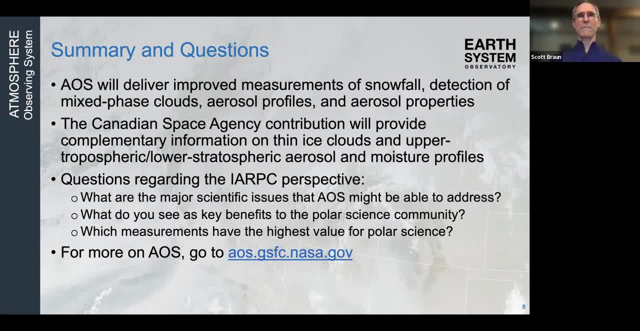 want to have gaps globally, um, but you know you might not want your revisit rate to be too long either. so that's one of the things that we're still looking at here, and trade it in phase a is what the the best timing is for a repeat cycle of those observations. but i think, if i recall, 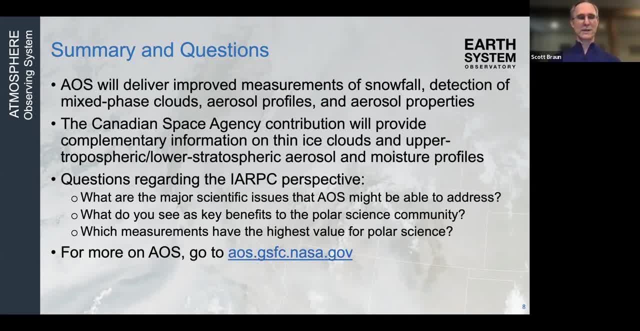 correctly. cloud satin, calypso are about two weeks for their repeat cycle and we might, it's better in the arctic, right, um, right, yeah, i mean how many? it's 90 minutes per orbit in a polar orbit, and so how many times i, how many times a day? is that? that's um. 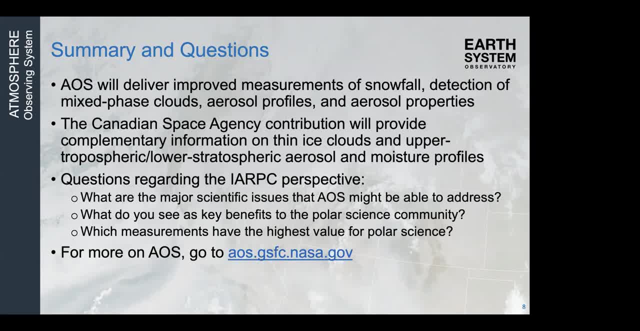 19 or something, 16 or 17 a day. it seems like, yeah, it's about that. yeah, i want to say it was like 15 or or 16 or so. yeah, so we'll have really good coverage in the arctic, um, compared to everywhere. 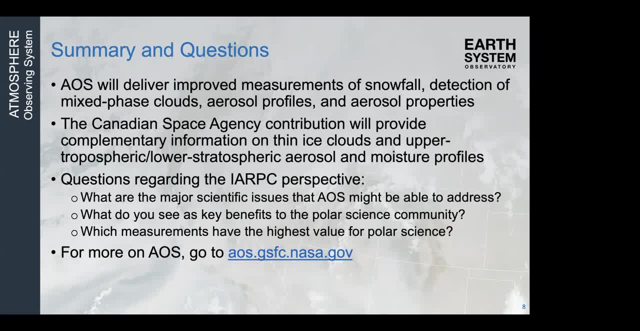 else it. it is a function of latitude, isn't it? yes, so the highest latitude you go to has a lot of coverage, you know. and as you slack off, let's take to 70 north. you've got i don't know. every few days, i would think something like that. 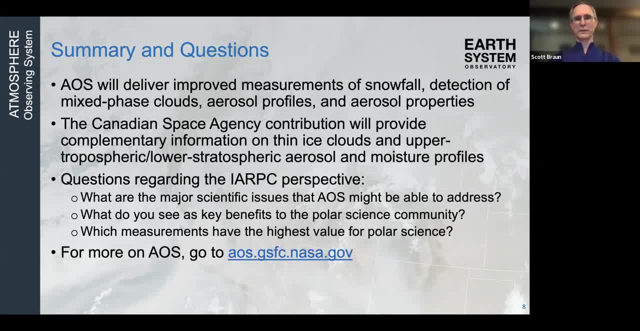 yeah, i think our biggest problems will be down in the tropics when we're trying to look at tropical convection um, and we're more likely to have larger gaps down in those regions. okay, so i was just curious. uh, it seemed like you're hinting that hsrl is coming out of langley and 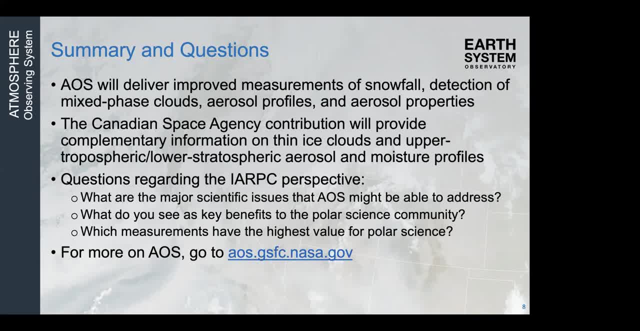 polar emitter is a goddard instrument. is that correct, or are these things still not decided until you get past phase eight? so we expect the passive instruments, the radiometer, the, the passive microwave radiometer and the polarimeter to be competed to industry, and the lidar at this point may be a hybrid of langley and competed um we, we haven't. 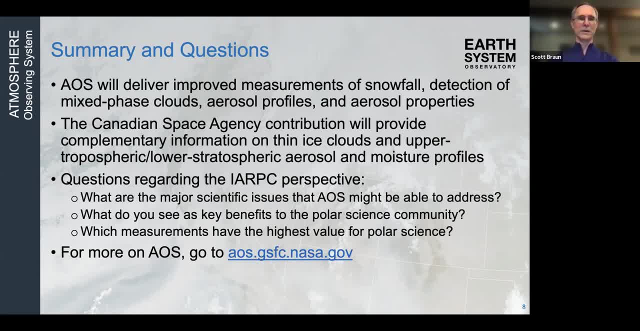 yet had our acquisition strategy meeting with headquarters to determine the best path forward for acquiring things. so certain instruments are directed the, the jp. we suspect that the, the polar radar will go to jpl, the inclined lidar will go to goddard. um, i'm trying to remember, uh, some of. 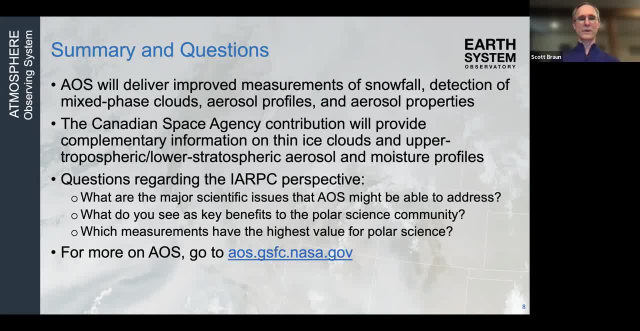 the others, the um, we have the, the contributed instruments from other um uh countries, and so most, most of the passives are going to be competed, and that was really the desire of headquarters: was to compete as much to industry as possible unless the capabilities were so unique to. 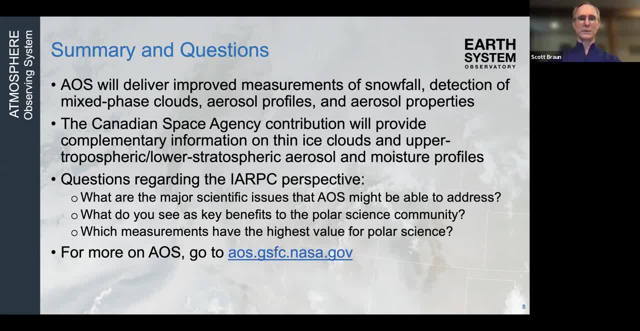 the nasa centers, or they were viewed as sort of tier one in terms of capabilities. just one question, scott. this is javier from uif. so hey, the, the microwave radiometers actually are direct detection or are in in? what's the name detection that i can't tell you? that's getting more into the engineering than i'm used to. 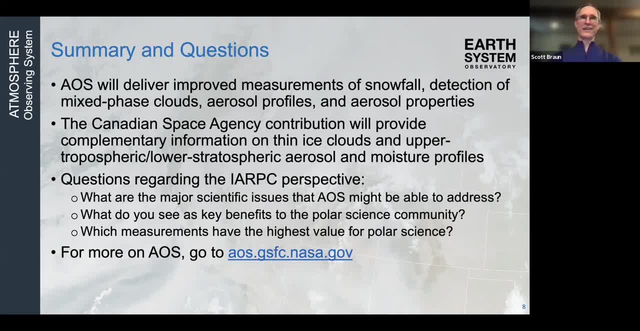 wondering. if i had our instrument scientists on here, i would be able to tell you right away, okay, well, so far. i mean, actually i have one microwave radiometer here sitting, but, um, what we have seen is, uh, um, changing the periodicity, if you, although current precipitation and changes significant changes in the intensity. 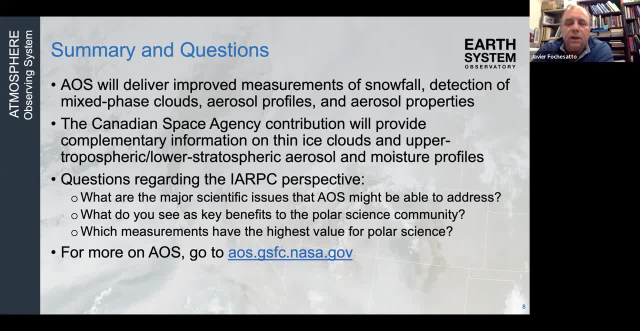 so changes in occurrence and changes in intensity, if, if you want some answer to those questions, that's what we have been seeing. so we are looking at, yeah, that's occurrence and intensity of what. oh, there's no precipitation. over how many years? well, i mean, uh, over the last uh, 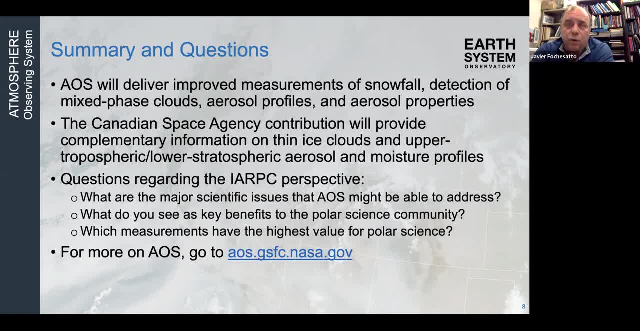 probably six years. we have seen warming events increasing, cyclonic advections and may eventually have been some other collected to some other, connected to some other lower latitudes, circulation patterns and eventually probably changes in the microphysical composition to actually trigger such tremendous precipitation events. here we have uh buildings that have collapsed in in fed państwa. 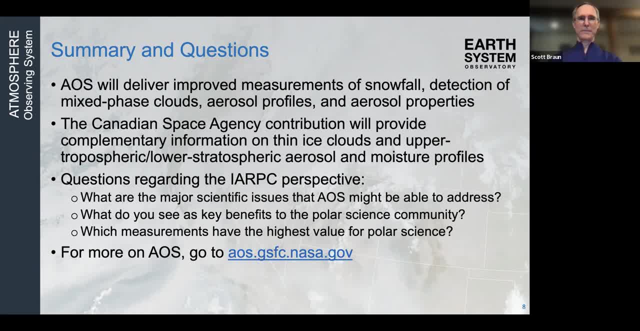 yeah, but yes, well, hey, here actually. yeah, one of the things that we wanted to do is provide some continuity with the a train. so we have the polar observatory, uh, having the same equatorial crosstime as cloud set and calypso, so that at least to some extent, the two records 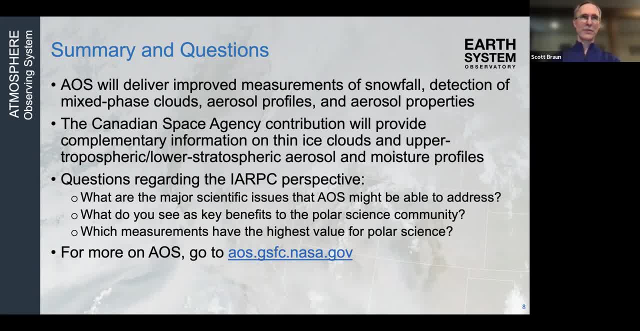 can be combined to look at some of the trends. you know they're not going to be exactly the same in terms of the measurements, but непosing to me. if you're looking for some sort of iceberg formation of the네 and enterprise to the end, do in that case deep d drivers needs to try to take out nice, so we are hoping that we will. After all, I can't see they're driving that way. but if there are any people trying toiero a single jet, jet is more the service tire for the airways in the A train time, so we knew about that. 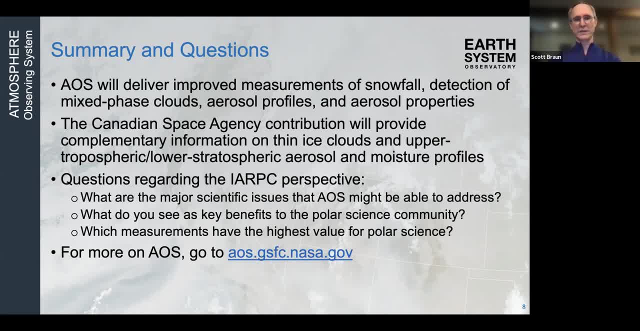 Hopefully it allows for some characterization of these trends. Yeah, Yep, Great. I had a question about the cloud phase which, since you asked about some of the major scientific issues and how important they are, I mean to me that's a really important one. 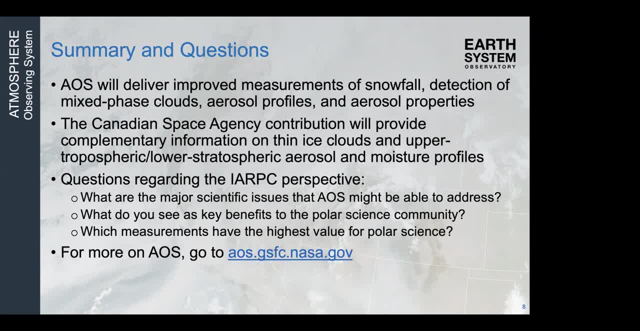 It's a really large uncertainty in the climate models, And so I was curious whether the new instruments how well they're going to be able to differentiate between phases compared to the instruments now. So with the LIDAR, it'll probably be comparable to Calypso in terms of its ability to identify the super cold liquid water at cloud top. 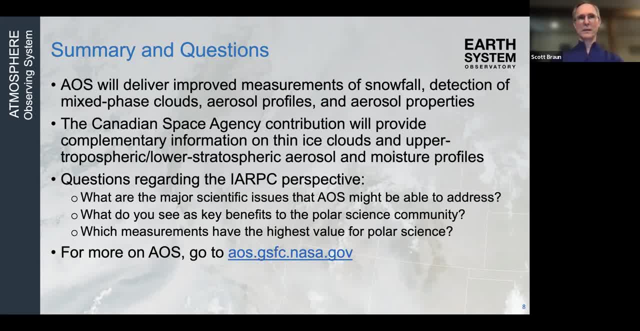 If you can't penetrate the cloud, you're not going to see further in. but it'll at least have comparable capability there And I don't think that the SNR will make as much of a difference as it does for aerosols. The polarimeter likely adds information because cloud top particle phase it will be one of the parameters that they can derive. 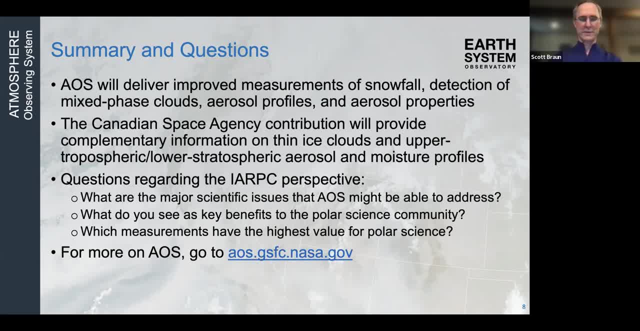 Again, it's kind of limited to cloud top. It's just difficult to determine phase deeper into the cloud. But at least the polarimeter will give you some sense of the spatially varying pattern of cloud phase And I think that's a really important thing. 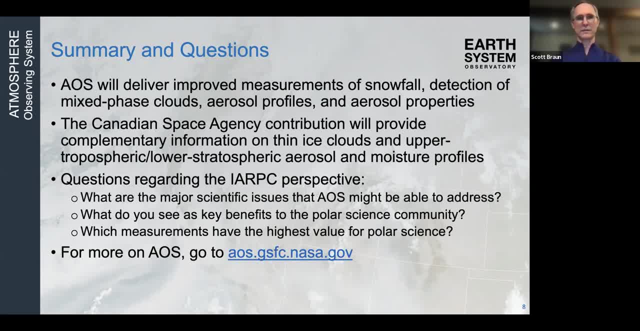 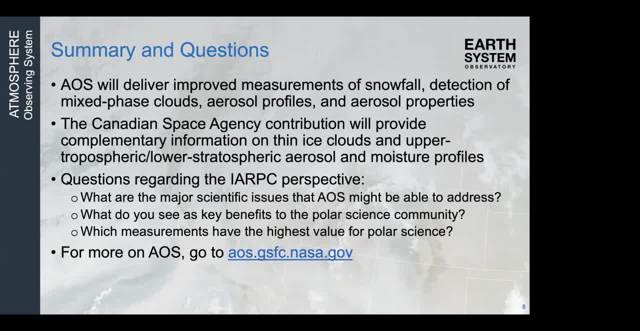 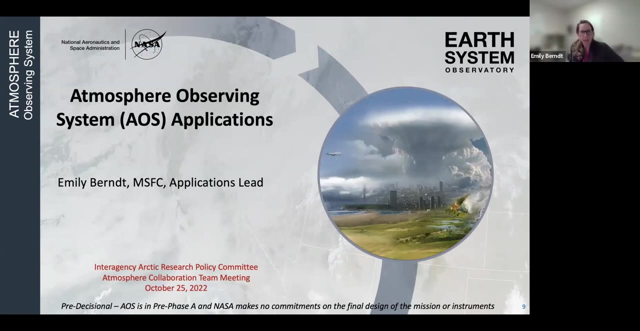 Thanks. All right, So we can move on to applications with Emily And then, if there's additional questions after her, we can continue the discussion. So next up is Emily. All right, So I'm Emily Barron. I'm at NASA Marshall Space Flight Center down in Huntsville. 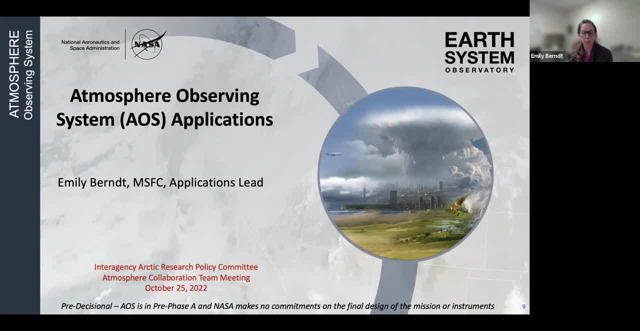 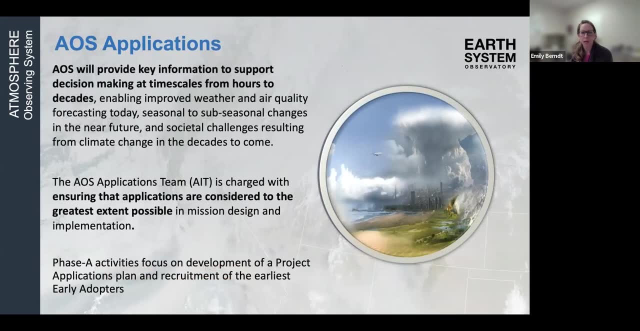 Alabama and I work within the Short-Term Prediction Research and Transition Center. Okay, so go ahead to the next slide. So what is AOS Applications? So we have something called the Applications Impact Team that we actually started at the same time as the science team. 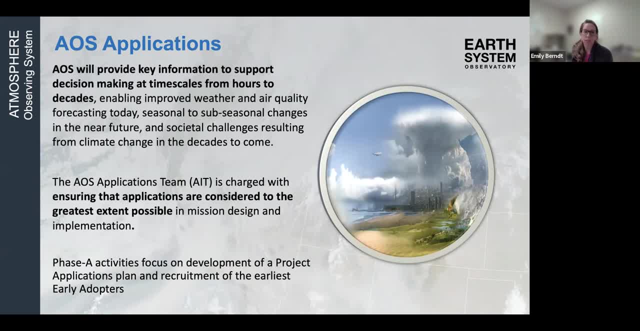 and participated in the mission study so that we could look at potential enabled applications. So, as the science team was coming up with architectures and potential geophysical variables that would be available, we considered those and used our expertise in applications to come up with some ideas about how the data could be used for societal applications. 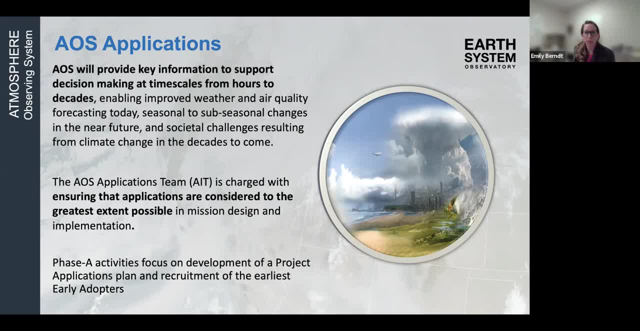 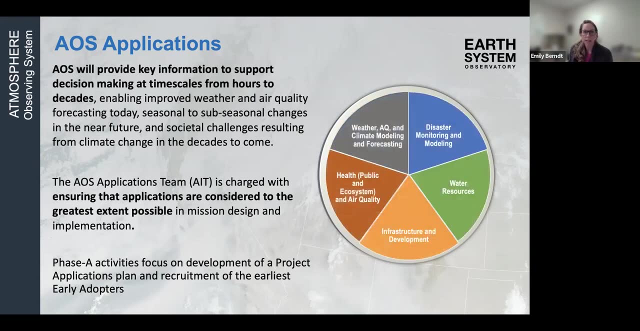 So a lot of it focuses around improving weather and air quality, forecasting seasonal to sub-seasonal changes in the future and societal changes resulting from climate change. You can press the space, bar, Scott. So here's our high-level thematic areas where we have applications. So disaster monitoring and 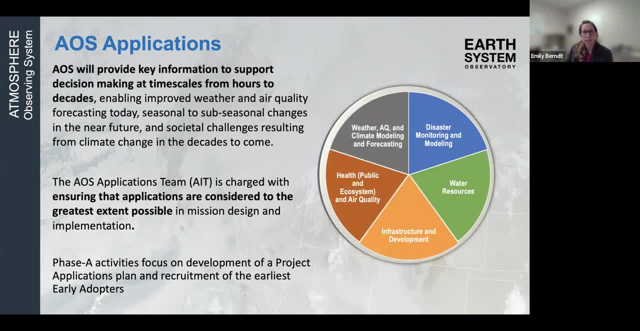 modeling. So I think a lot of precip-driven types of applications, such as landslides, also atmospheric type of disasters, such as wildfires, volcanic smoke, tracking, smoke, water resources, infrastructure and development, health and air quality, and then 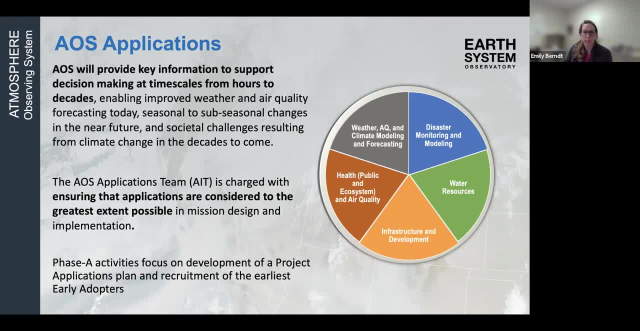 of course, the weather, air quality and climate modeling and forecasting. So in the current phase, in phase A, we're focusing on the development of project applications plan, meaning, how are we going to carry out applications and engage with stakeholders throughout the mission life and? 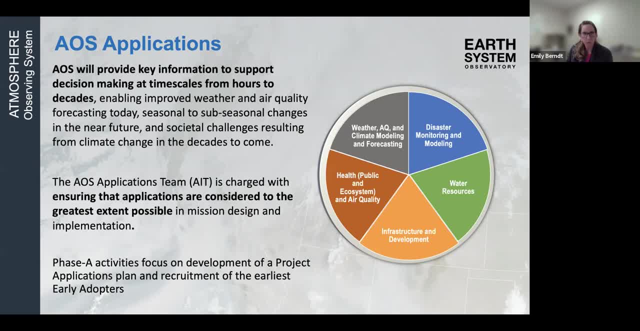 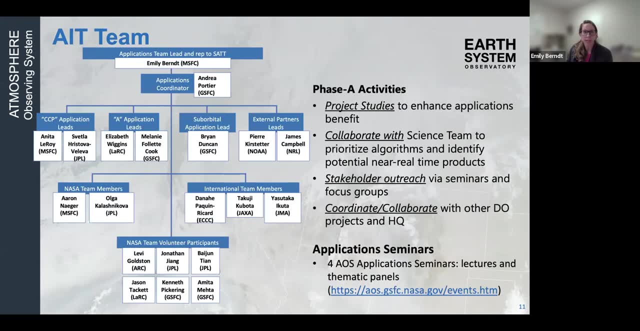 starting to recruit early adopters. You can go to the next slide. Typically, early adopters are people who are interested in using the data or proxy data prior to launch, So we have a wide range of people who participate in the applications impact team across NASA centers. 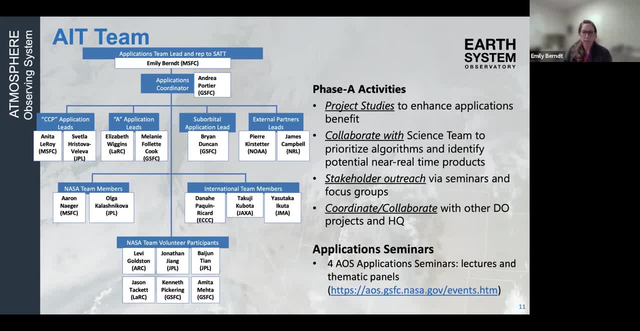 with experience in aerosols and experience in weather type of applications. So we do project studies to enhance applications. So looking at latency, engaging stakeholders on what their needs are for data formats and ideas that they have for applications. We collaborate with the science team to help prioritize algorithms and identify potential. 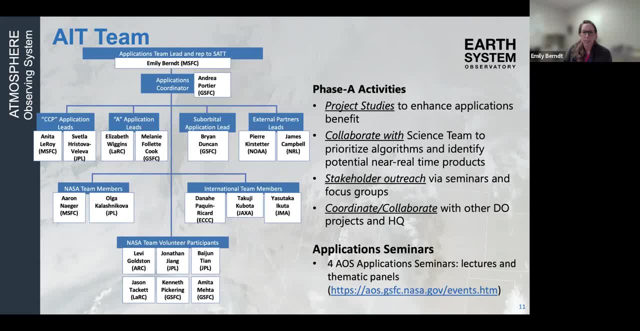 products and stakeholder outreach. So we have seminars and we have focus groups that we conduct and we collaborate with the other DO projects, the other missions that are expected to launch around the same time period period and headquarters. There's a link to some of the application seminars if you're interested. 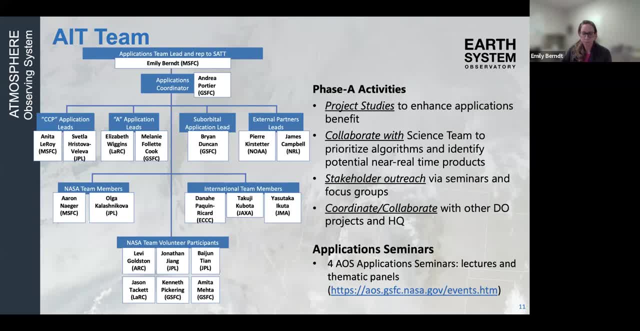 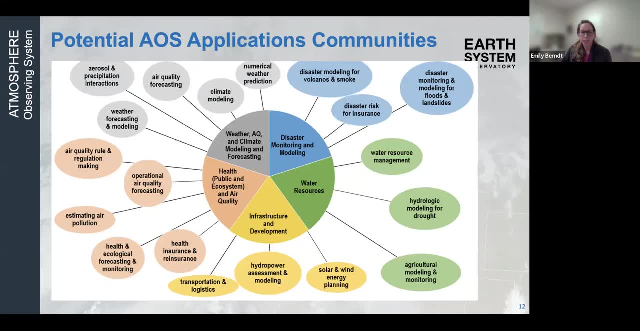 in looking back at some of those and what we've covered. Next slide, please. Okay, so under each of our thematic areas there you can see we have a chart of a little bit more specific applications. We actually identified something like 70 potential applications and then we kind of paired it down. 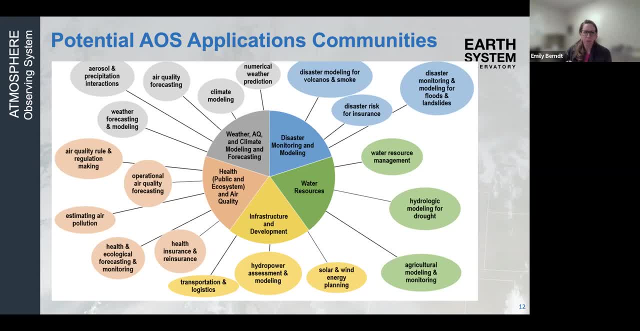 and grouped them to areas of maybe about 25, 26 within our five areas, So you can see some potential areas that may interest you, maybe related to air quality and aerosols and weather forecasting or climate modeling or some of the disaster type of events that occur. 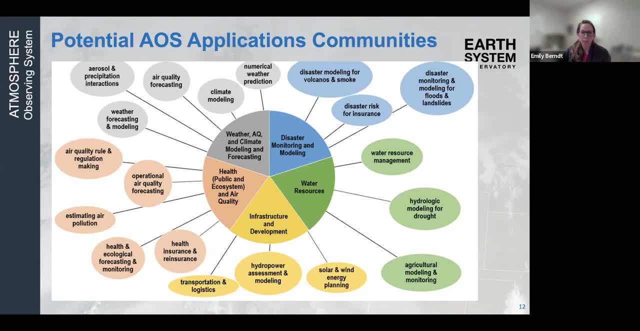 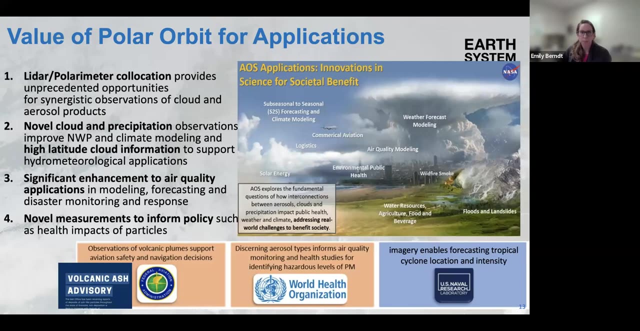 within the Arctic, especially around fires and volcanoes, and also with hydrology and some of the landslides, Modeling and risk. You can go to the next slide, So I included this slide for the value of the applications related to the polar orbiting architecture. I have a backup slide for the 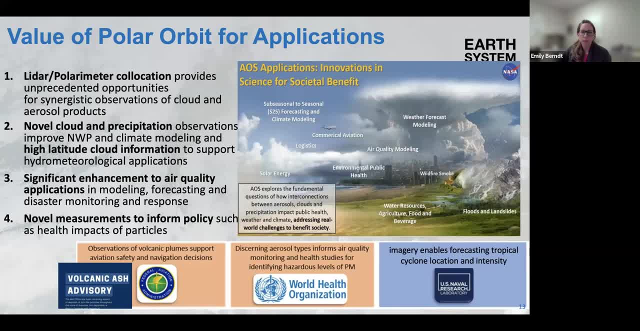 inclined but figured, I would just focus in here. So one of the things that we are looking forward to is the co-location of the LIDAR and polarimeter to provide opportunities for synergistic observations of cloud and air. So we're going to be looking at the LIDAR and polarimeter. 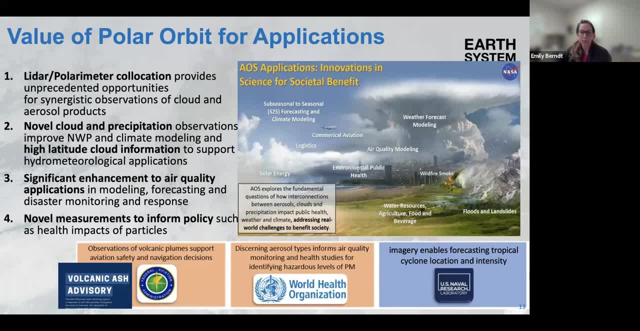 and Generally subpar and you'll see I will put a FAQ. You may have touched on the Tara dive material as well And it's sort of an forthcoming timeline in terms of softwares and other amós or household objects related to Microsoft. может take off for wind and aerosol products to 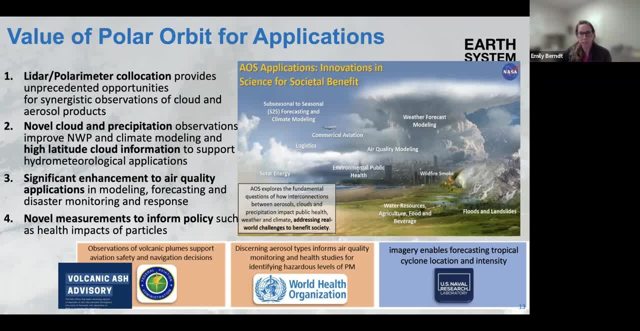 get some of the context information and also some of the vertical information. There's a lot of users who would really benefit from more information in the vertical to help them make decisions, whether it's the aviation community, related to air traffic and tracking, hazards, or within weather forecasting. 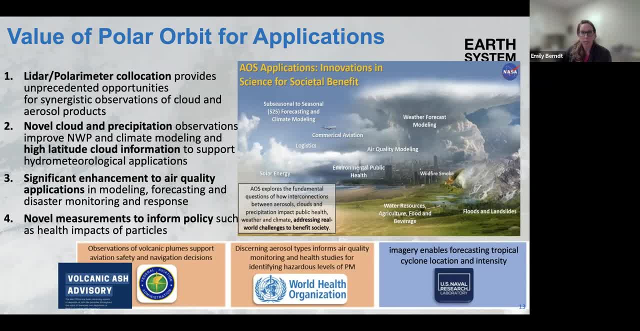 A lot of focus because a lot of the instruments are more named and the instruments start withir patches blue, So that should be an input, I think, for OK, great, Thank you, Ray. Thanks, radar, pointing with not a lot of context. a lot of focus revolves around some of the 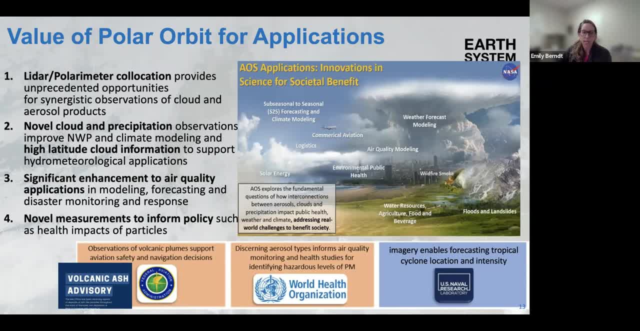 improvements to numerical weather prediction and climate modeling, that the data can be really valuable for improving models, developing parameterizations and validating models also. So we do have quite a few early stakeholders that we have engaged with around this type of application and area. 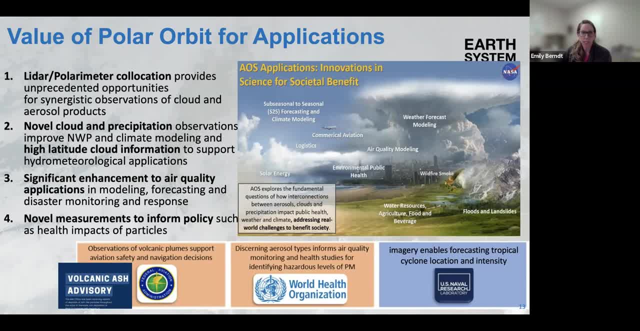 We're looking forward to enhancement to air quality applications and modeling and forecasting, and disaster monitoring and response, and novel measurements that inform policy, such as health impacts and particles. So we just have a few examples there that range from engaging with volcanic ash advisory centers. 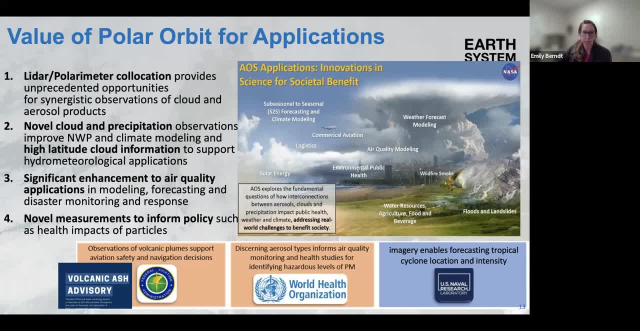 We've had a couple engagements with them And some of the international DACs to working with NRL and improving tropical cyclone forecasting of location intensity, that the passive microwave radiometers are really important for that Let's see. And that's my last slide. 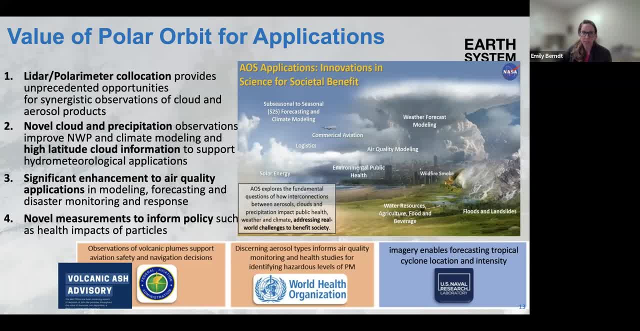 So if there's any questions that you have, if there's any applications ideas, and especially if you have ideas that you have a science idea and you feel like there's an application or a product that could be developed and flow out Out of that application idea, we're interested to hear those. 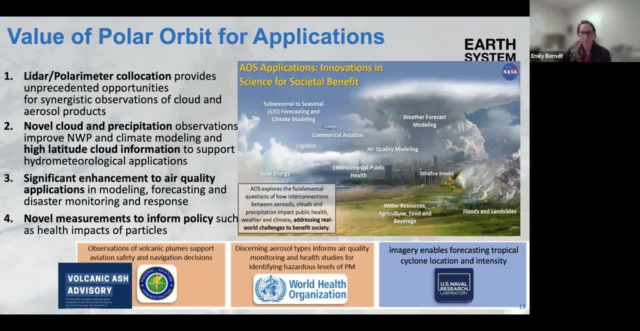 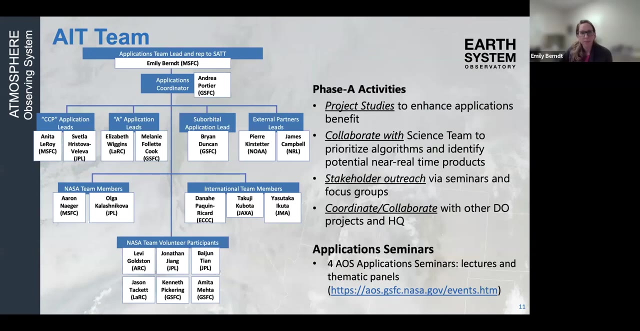 Jack, do you want to go ahead and ask your question? I was just wondering if you could back up to that slide that told the people that were already engaged in your planning: Yeah, Go ahead. Yeah, So I'm just. I'm not seeing anybody on that list that seems terribly interested in Arctic. 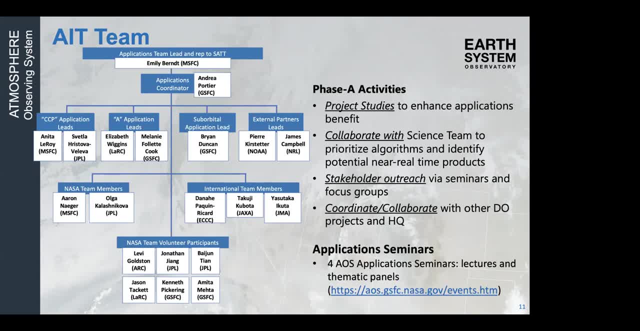 issues- And there are a lot of pressing ones- And the fact that you're going to get much better coverage at high latitudes than anywhere else seems that maybe there ought to be someone, maybe someone on this call that'd be somehow involved in this, because, I mean, all of your examples are great and they're good for society. 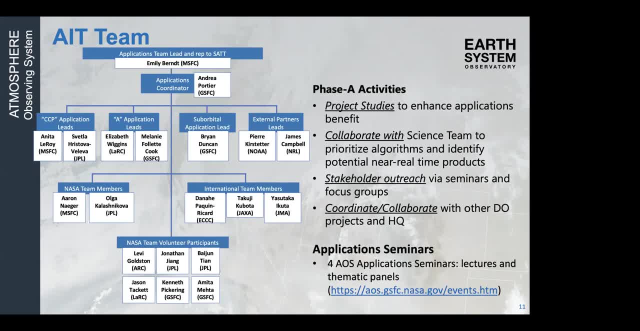 and everything, But I think the issues in the Arctic, I think, are quite a bit different. We heard already about the mixed-phase cloud and surface energy balance, and how fast is all that ice going to melt? right, And what can you tell us by the role of clouds and surface energy balance? 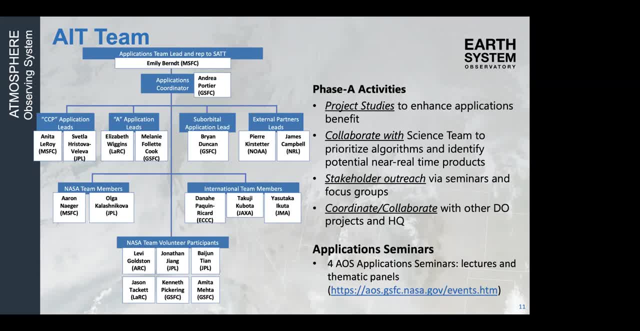 And I think this platform, this AOS, could tell a lot, but there's nobody advocating on your team here to really focus on any of that. Yeah, I think we've had some champions here and there. Yeah, I could tell you the data's really great. 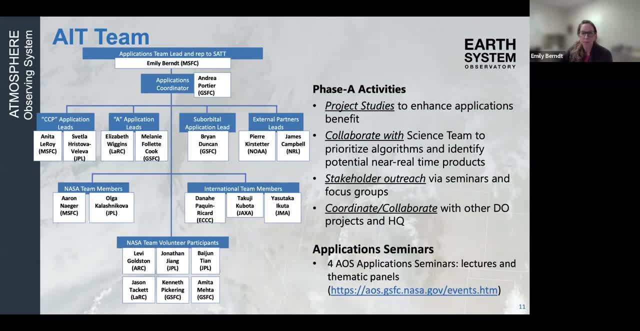 We're working on a lot of this over the last year or so And it's been really exciting. It's been interesting And I think that's been a very, very good example of where there's been a lot of advocate for being able to look at fires and biomass burning and consideration for how high the 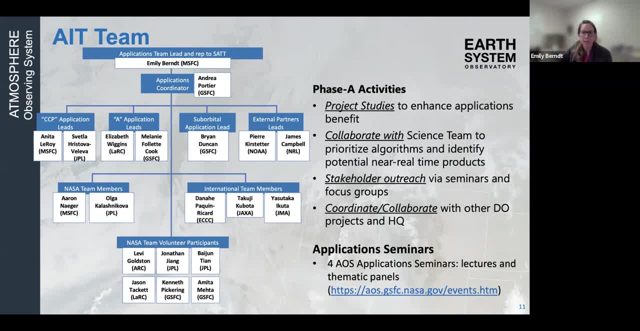 inclined orbit would go for us to be able to do that. Within the organization that I work in, we've had engagements with the Alaska National Weather Service and they use some of the GPM precipitation products very heavily. Maybe Brian is on here and can speak. 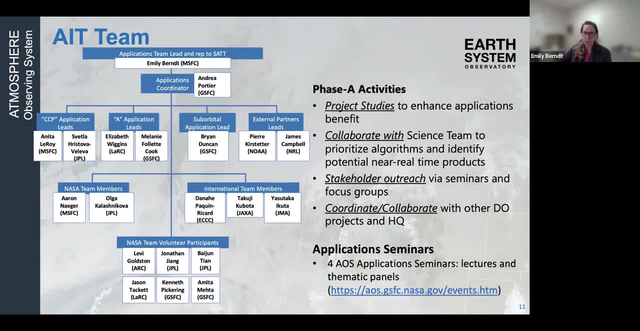 on here and can speak. you know we're. we definitely welcome more input. you know we're. we're also in the process of revising our applications traceability matrix, and so if there's input on how to better represent arctic type of applications, we're open to that right. well, 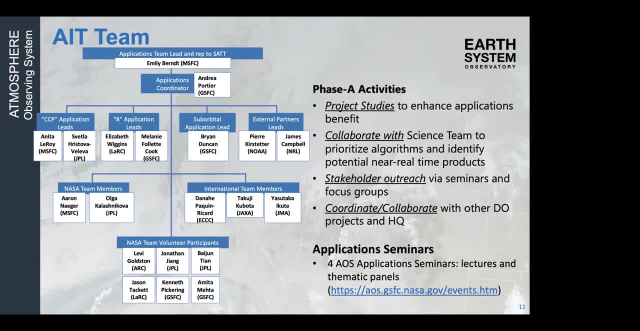 it'd be great to hear from brian, but i was thinking that you know javier or david brown which might speak to. that also was more expertise than i could. so if anybody's got any comments out of those three at least, or anybody else, looks like, yeah, i have a comment, but it's maybe. it's not like a direct response. so 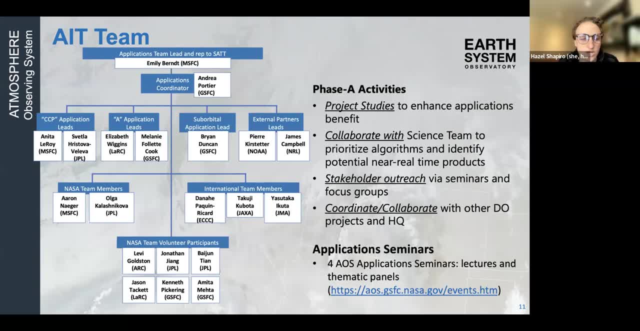 brian, or if others want to speak directly to jack's question, go ahead. yes, this is brian duncan. yeah, we i. i think that emily really hit the nail on the head is we didn't know what the orbits would actually be and what, until, uh, rather recently. so this is. 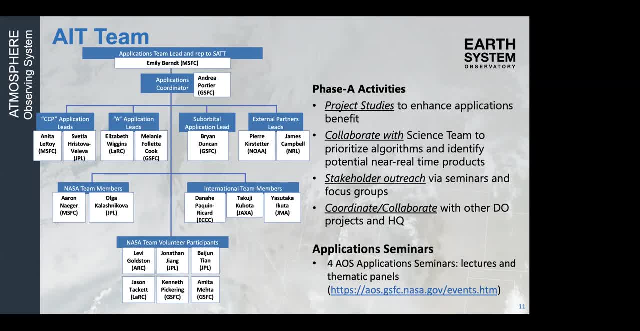 an issue we need to revisit, definitely, and i'm um and i'll definitely be bringing this up at the next uh application impact team. call you. Yeah, we, i mean we have a copy of our atm on the uh web page. that, uh, that's listed down there, not the events web page, but if you go to the main site that you know we're happy. 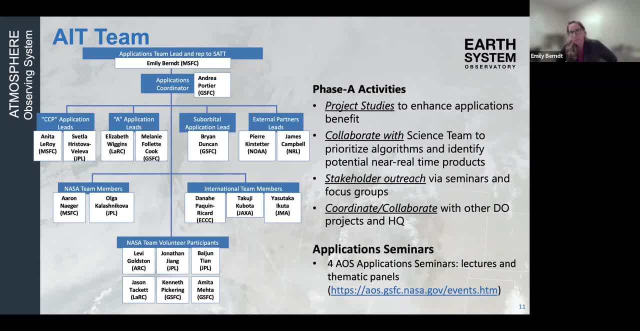 to have some of you take a look at it and what we have represented and provide any feedback on anything that we're missing. so, emily, this is david, again being irritating. um, so we've got a little bit of a flow through here we've got. we've got a couple of questions. 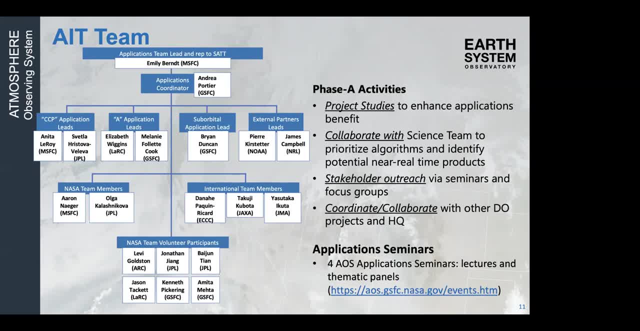 that we're trying to get across um. one part is specifically about the points and donc um to get arctic expertise, uh, you probably have a fair amount from the canadian space agency, so can you talk about the links? you know how close that is um for their interests. 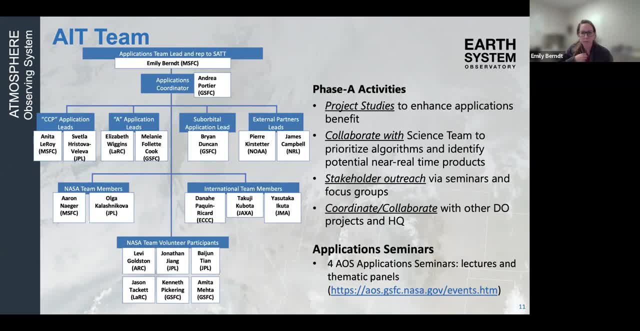 and so on, um, so we do have one member from environment Canada, Donna Haye. um, she is more of a modeler, um, in kind of her background as a freelancer, she does a lot ofängthe things like, um, well, like this way. and so we have a third point about her being an astronaut, and she has a 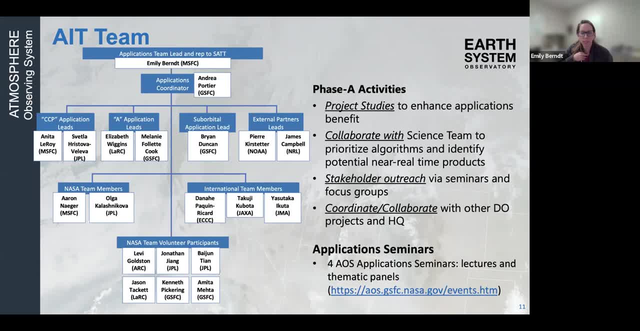 of her application interest area is more related to using the data to approve models. Okay, I guess, Emily, we could reach out to folks at CSA and just double check whether there are additional people who might be able to help with applications. One really good piece of news we got just recently was that 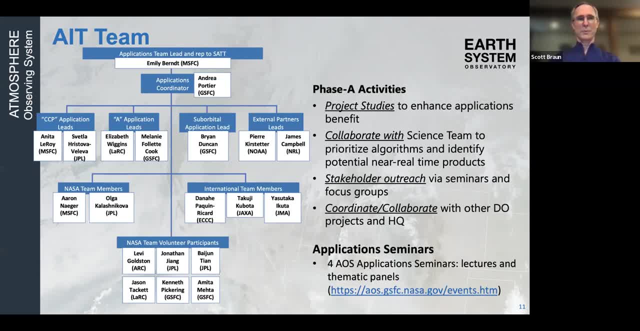 CSA announced that they had secured the funding for their portion of the mission, so we're really happy to hear that. I don't know if that means that they're also able to then start funding people on the application side that maybe were volunteering before, so it might be a good time to revisit with them. 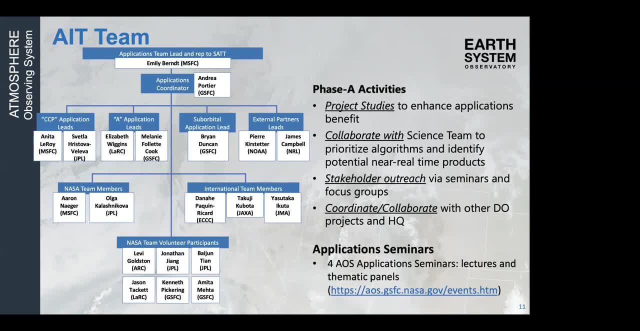 Thanks for the presentations. They were really interesting and I'm not a technical expert on any of these topics. but I just noticed in some of the places where you're looking for crossover applications, a lot of those have a really direct tie to IRBIC's next five. 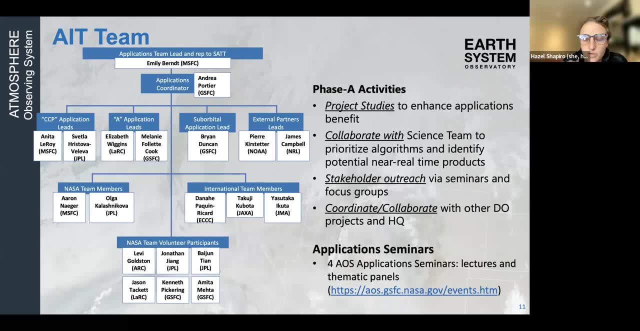 year plan, Which has is going to be developing these priority area groups around things like disaster mitigation and response and human health, in addition to working with some of these like climate modeling and stuff like that, And so I don't have a direct like follow up action. 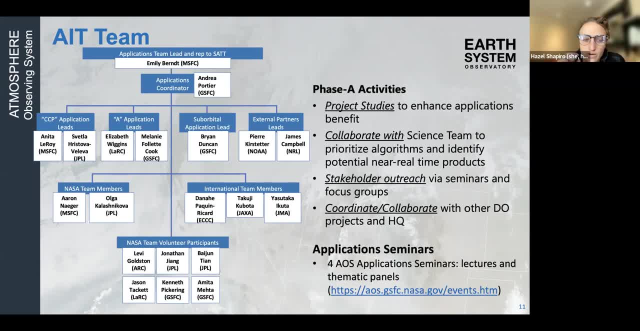 But we're going to be moving from like having a plan to starting to implement that in the next couple of weeks and I think that this would be a really interesting thing For the atmosphere team to carry forward or for the AOS group to stay involved with IRBIC and see if there is some way that we can help you answer some of those questions. 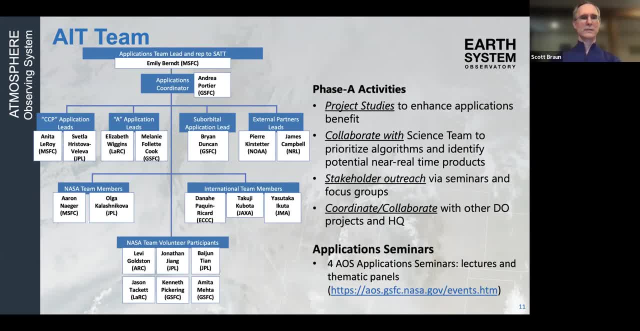 Yeah, we certainly have. to the extent Brian is able to participate in some of the IRBIC activities, He could be one of our key links to the community, to kind of learn how we can connect at this speed, If we have the time to do that. 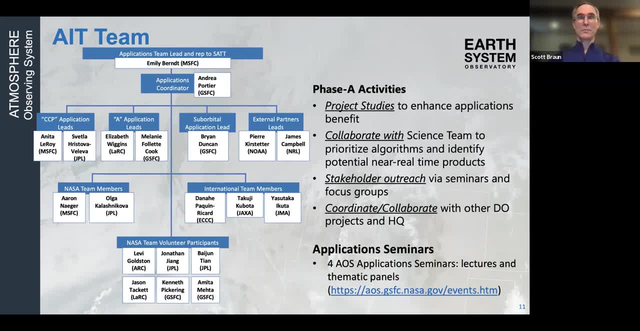 Yeah, Thank you, Thanks, Thanks, Thanks, Thanks, Thanks. somebody on the science side who would be able to connect as well and look into that? so could i? could i ask? um, this is david again. uh, i got many questions, um, so one the, it seems like, uh, your. 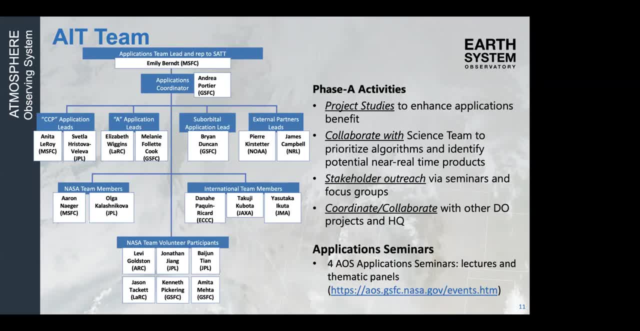 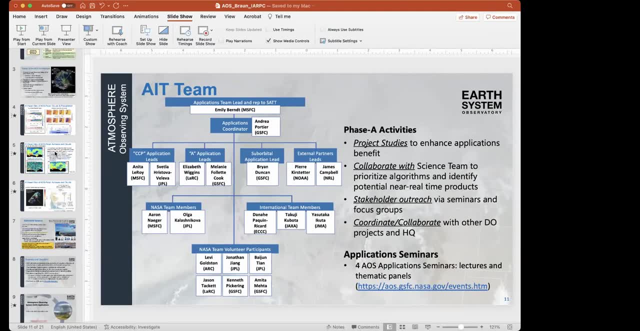 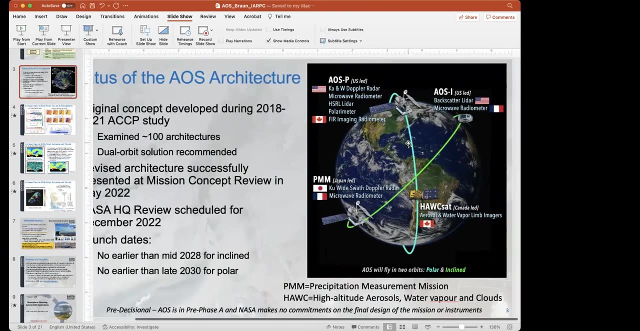 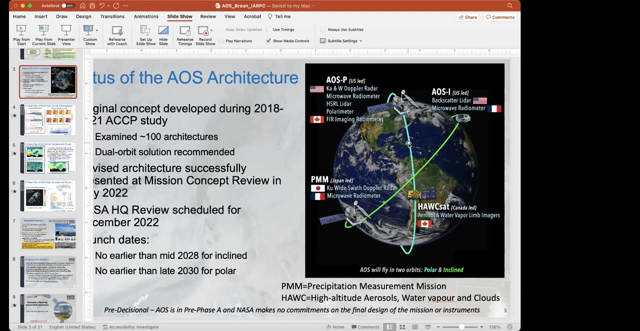 satellite, the polar satellite, is in some ways a follow-on to cloudsat and calypso um, and i think they've really done a lot with you know their products to make them available. so can you talk a little bit? maybe it's early, uh, in relation to what you plan to do, but 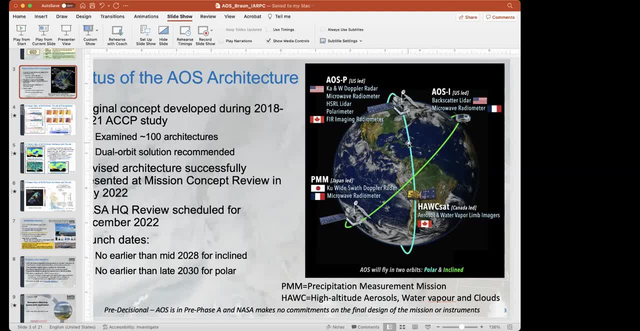 maybe talk a little bit about that aspect of it which, uh, you know, gets it out to the broader scientific community. yeah, so you know, with this mission we emphasized fairly early on that, you know, applications was uh really important along with the science, whereas a lot of missions in the past might have started with the science and the applications kind. 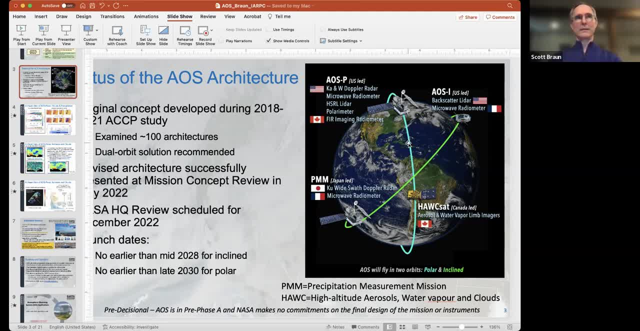 of came along later. so we we actually did a study looking at data latency, uh, to see what we you know, to be able to identify some realistic uh requirements on getting data to the ground and out to users. um, i think there's a fair bit of it that we can get down and i don't have the 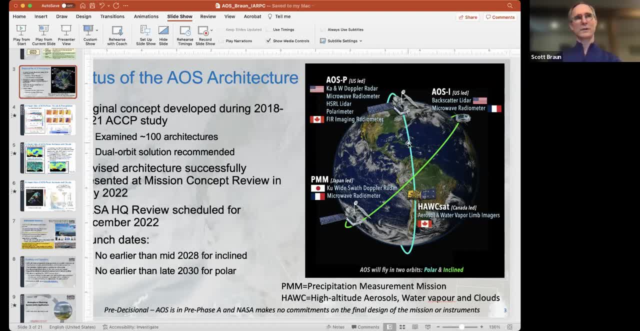 numbers off the top of my head. we set certain targets for a certain fraction of the data within three hours, a larger fraction within four or five hours, and so on. um and some of the the algorithm team, some of the algorithms kind of um, naturally you know, work well for applications. you. 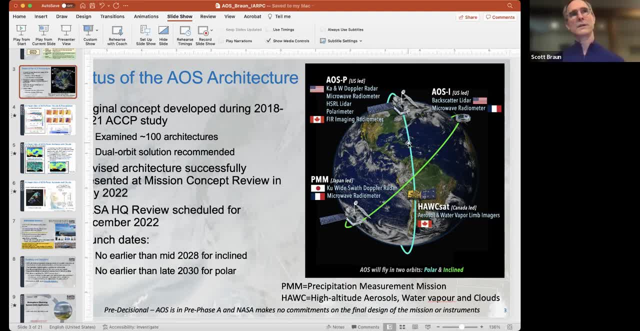 can get them out real quick with some of the sensors it. it might be a little bit more challenging, like the lidars, and what they tend to try to do is, um, to do an early version of the product. that might bring in an analysis instead of some kind of a. 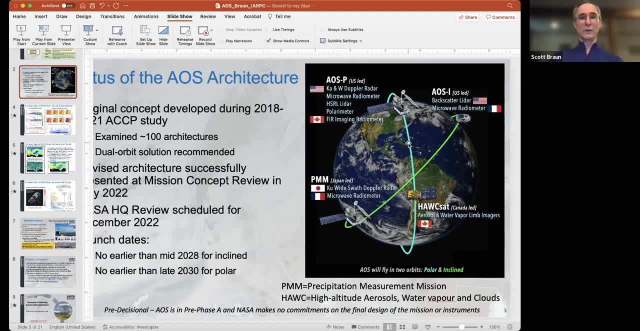 ledger or some other observations to help get an early estimate of aerosol properties, uh, to be followed up later with with one that's using maybe the more climate quality type of measurement. but the goal will certainly be to try to get some real-time uh data out as well as. 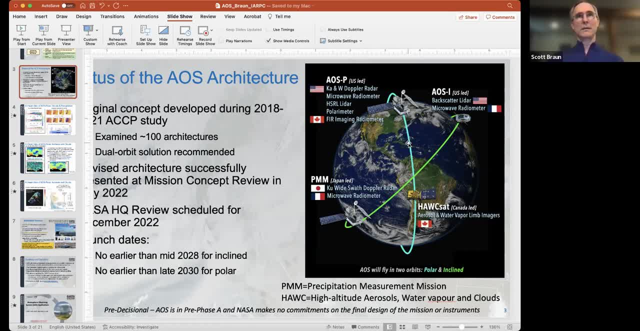 the climate quality type products, uh, and we also expect that these all the data or the data management will follow. nasa's is open science policy that they're developing now, And so all of the missions are expected to adopt to open science. So both for the products as well as I think, 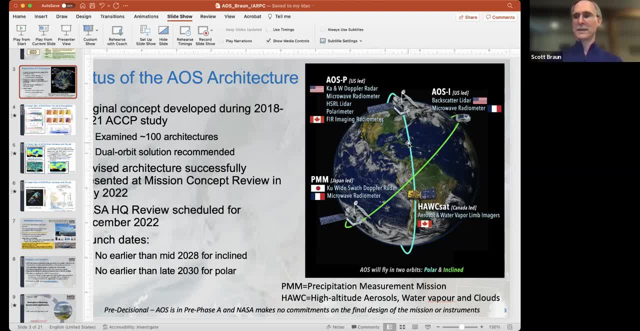 even the algorithms, and that's something that's it's in development. We're working with headquarters to figure out how all that gets implemented. And a lot of these data sets, not only ours but from the other designated observable missions, will probably be on some earth data cloud. 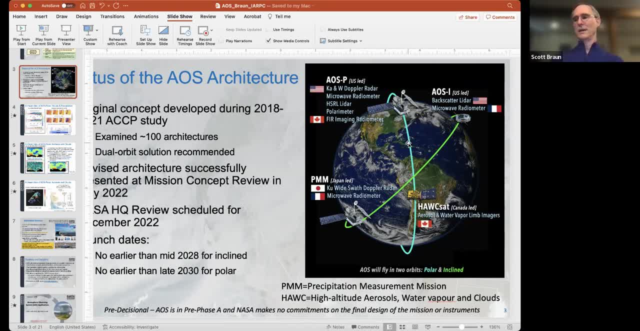 that allows for ready access of all the data sets, But we are still fairly early and we'll kind of define that more as we go forward. Thank you, Yeah, and as we engage with communities, one of the things that we can ask them about is preferred formats, preferred visualizations. 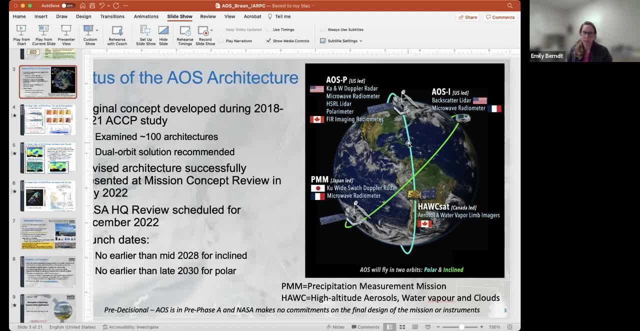 And there's a pretty large range of users where you have very sophisticated users who are more modeling agencies or university researchers that can handle the net CDF data. But one of the things that headquarters had us do is look for some users that were non-traditional type of users. 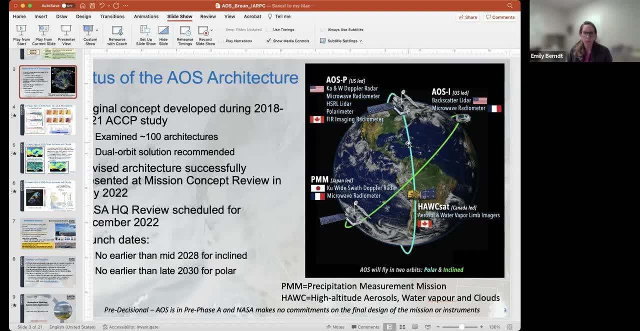 in industry and private company, And so one of the things to anticipate is working with those types of users is providing gridded level three, level four products or visualizations that they can use pretty easily And you use on hand. So those are some of the things that we're thinking. 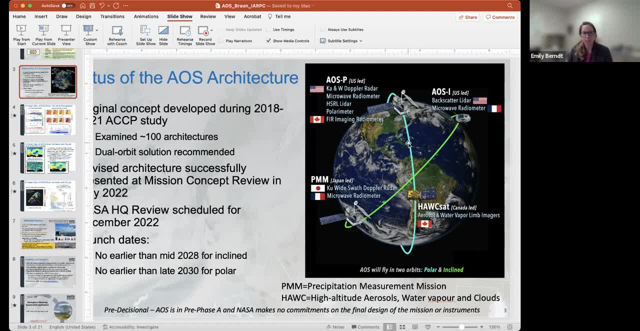 on the application side, as far as how to take the data and make it accessible and usable for users who aren't as familiar with it, And for those who might not be familiar with some of the terminology. level two would be your retrieved quantities in the orbital swaths. 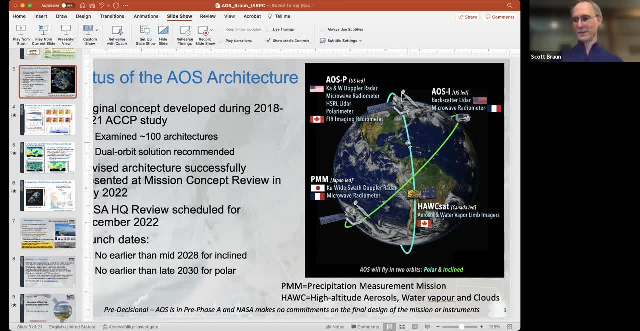 Level three is typically gridded to something standard grid. And level three is typically gridded to something standard grid. And then level four is assimilated products, where you assimilate the observations into the model And it's actually the resultant model fields. 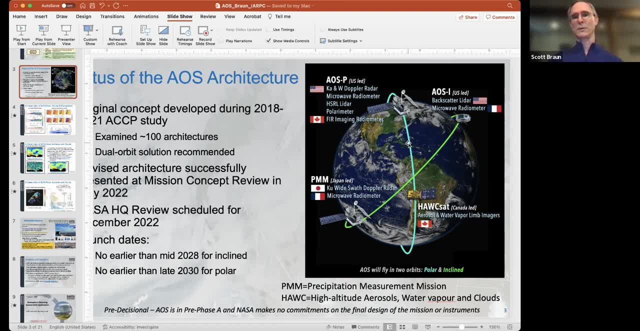 that get released as a product And we'll be working very closely with the Goddard Global Modeling and Assimilation Office to develop some of those assimilated products. Hey Scott, I just wanted to advertise that AOS will have a town hall at AGU and also at AMS. 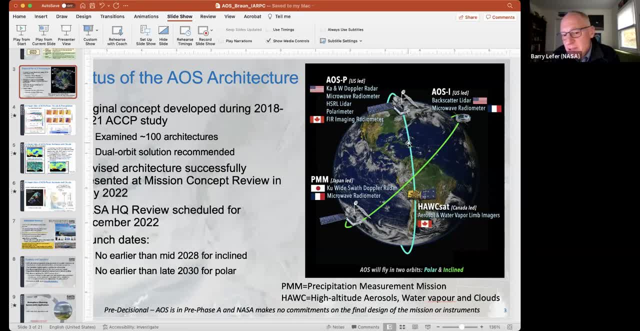 So that's a great place to go to get well, meet Scott and I will be there- but to meet more members of the science team and to hear more about AOS and to ask these questions. It'd be great to ask these questions again. 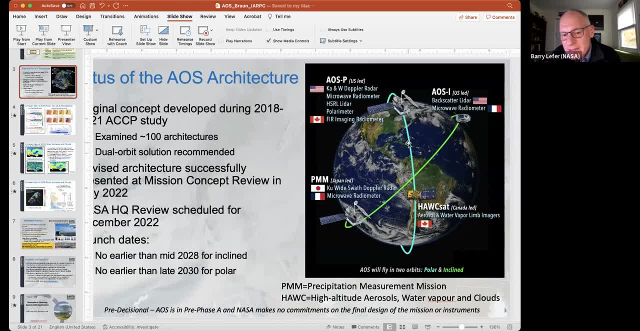 about Arctic applications, and maybe we'll have more information then about the orbit and how many, what the revisit time will be at different latitudes. So- Yeah, I'm not sure yet, but some other things might, And we'll also have every quarter. 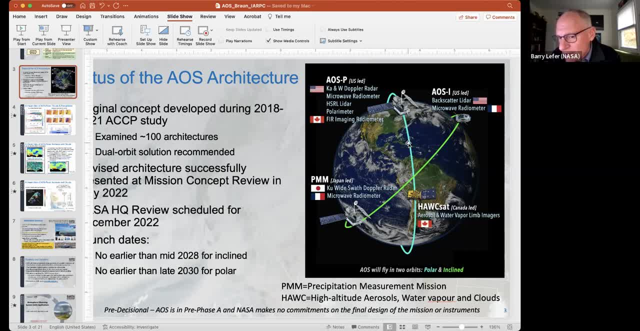 we have a community webinar, A community forum. We haven't actually. we might be due for one pretty soon. We have a mailing list for anybody interested in it. If you go to the webpage, you can find the link to join the community list. 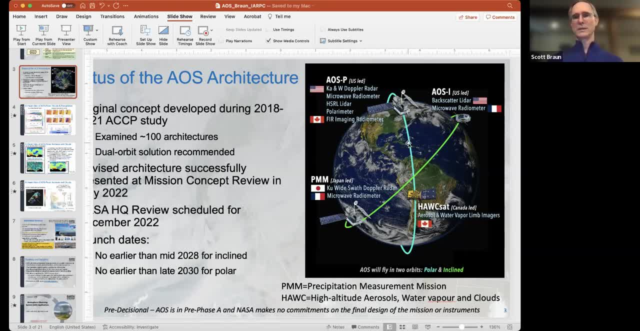 And so we try about once every quarter to just give the community an update on what's happening with the project on the science side, with the future procurements once, like if RFPs are gonna be released anytime soon and things of that sort. 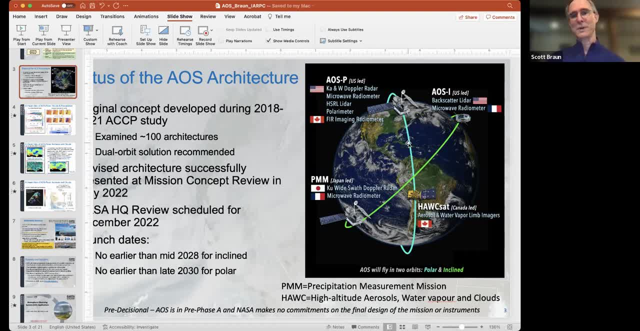 And I believe we're probably due in November. but I need to get it on the project management team's vision because I don't think they've been thinking about it lately And I think they're recorded And so you can see the last one. 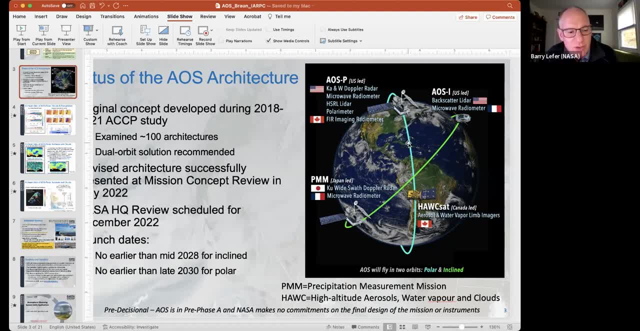 Or go back and see different ones if you want. So, but yeah, we- The ATU town hall isn't on the webpage yet. We just paid- a week or so- last Friday, I think- the fee to make it official that it's a town hall. 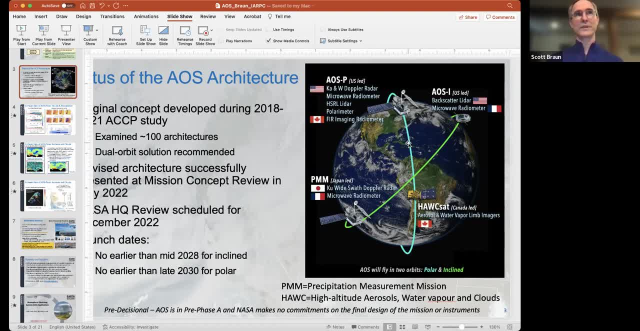 but it hasn't made it onto the webpage yet. And looking at the schedule for the AMS meeting- yet I don't really see much of. I saw the town hall identified among the list of town halls but I didn't see town halls actually in the schedule yet. 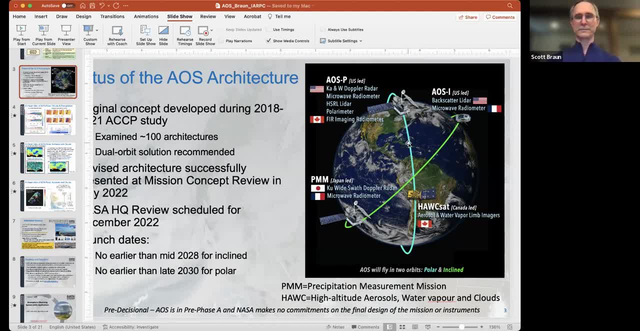 So yeah, But that might take a little bit longer before they show up. Well, thanks to Scott and Emily and thanks for the nice questions. Lauren, I saw you had your hand raised. Do you have a quick question? Just a super quick comment maybe for Emily. 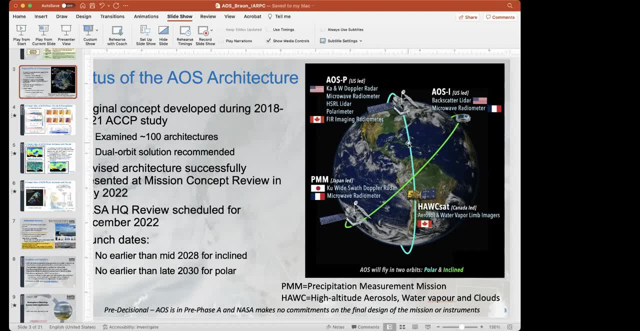 This is since you guys were talking about applications. I was just gonna say that, like Worldview is really great for educational purposes. I imagine this will be integrated, probably, with Worldview, but I give like periodic presentations to elementary schoolers, you know, for career day at school, and they use it and it's easy. 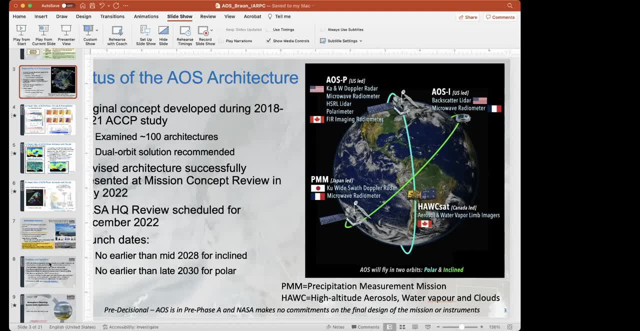 for even for elementary school students to use, and it's great. So you know that. you know if you could continue to integrate with that, that's a really great product. Yeah, I certainly hope that we'll continue to do that. I'd like to use Worldview for a lot of data sets, and it is a readily accessible way of. 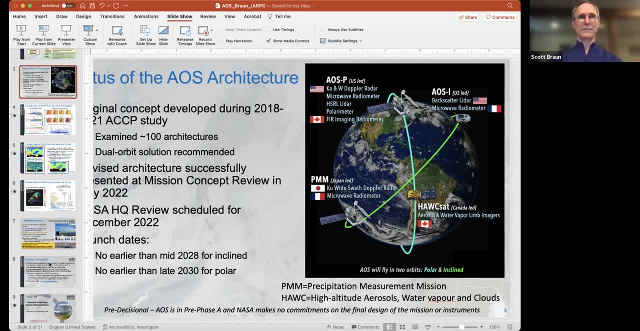 visualizing the data without having to download anything, And we will also, over time, produce a set of visualizations that could be used as teaching tools too. I mean, anytime you give a talk to a general audience, visualizations, animations, are. 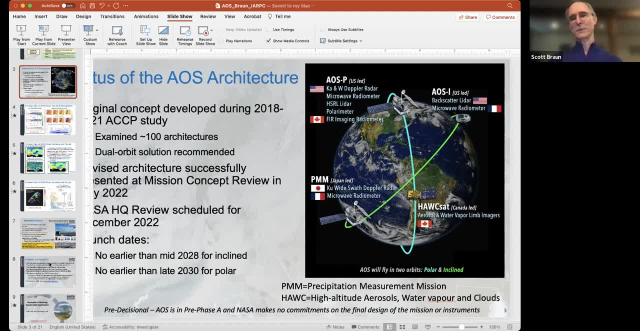 great to use and we hope over time to develop a good suite of visualizations to kind of characterize the science and the type of measurement. It's the synergy of the measurements and things of that sort. but it'll take some time to generate those pre-launch and then, once the mission's going, we'll hopefully generate